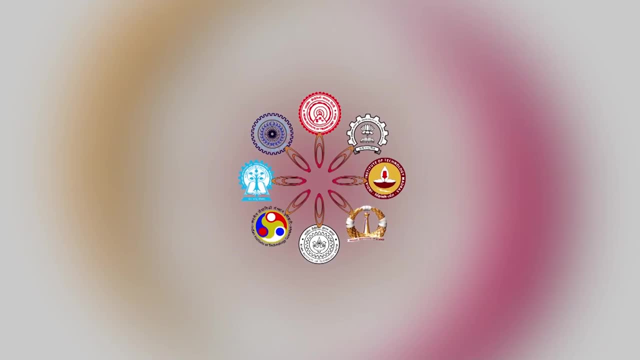 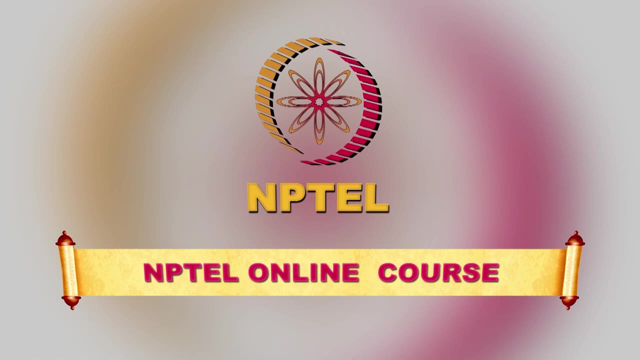 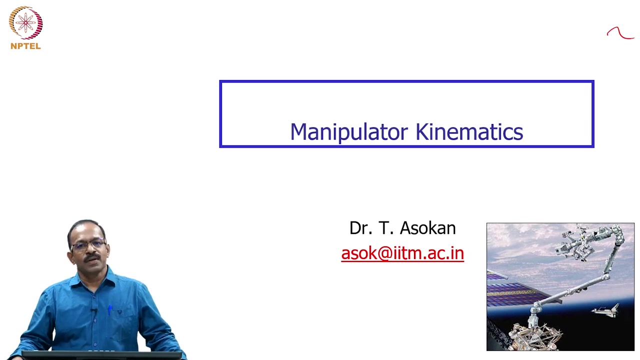 Very good morning. welcome back to this course on Introduction to Robotics. So we will start the topic Manipulator Kinematics today. In the last few classes I mentioned about the development of robotics in general and the applications of robotic technology in various fields, and I mentioned that industrial robotics is one of the major areas of robotics application. 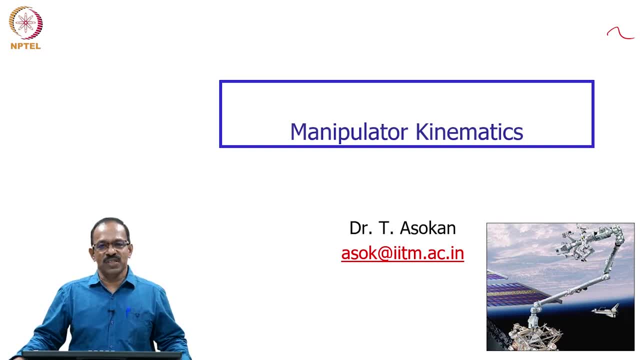 And when we discussed about the important topics in robotics, I mentioned that manipulator kinematics is one of the most important parts which any robotics engineer should need to understand, and then this will actually form the basis for learning robotics. in many other applications also, like field and service robotics. You need to have a basic understanding. 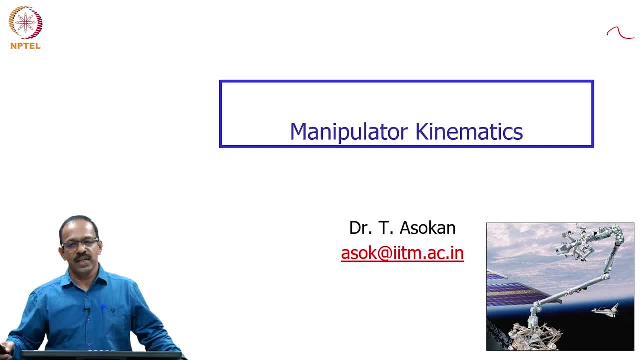 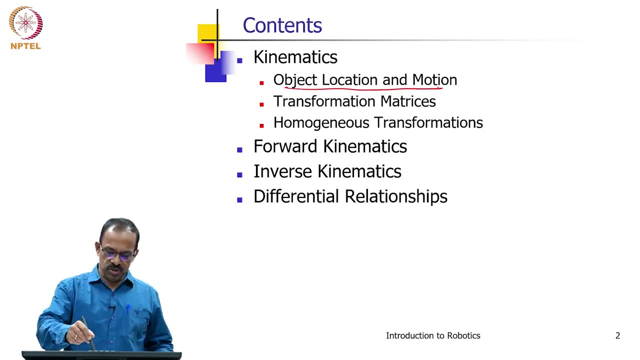 of manipulator kinematics. So we will be starting this discussion today And as part of this kinematics, we will be talking about the object, location and motion as the first step. So kinematics basically talks about the position and velocity relationships. 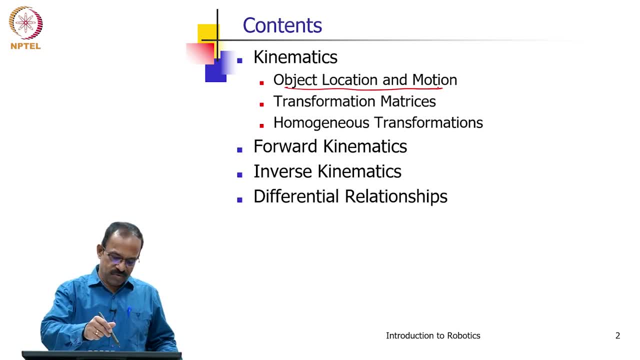 in robotics. So, in order to understand that, first we will talk about the object, location and motion, How do we actually represent an object in the 3D space and how do we actually represent the motion of an object in 3D space will be discussed, And then we will talk something. 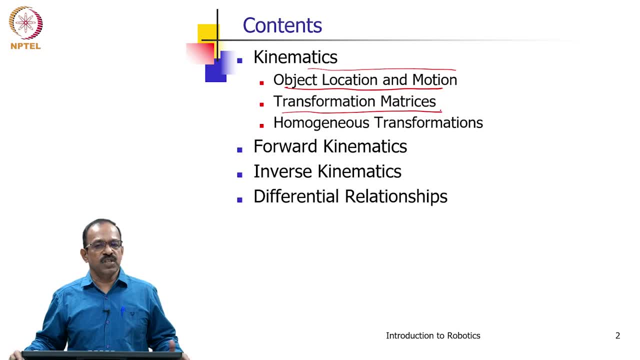 about the transformation matrices. So if an object is moving in the 3D space and when the movement includes the translation rotation, then how do we actually represent these transformations can be explained using transformation matrices. So we talk about transformation matrices and then we talk about something called homogeneous transformations. So to represent the object. 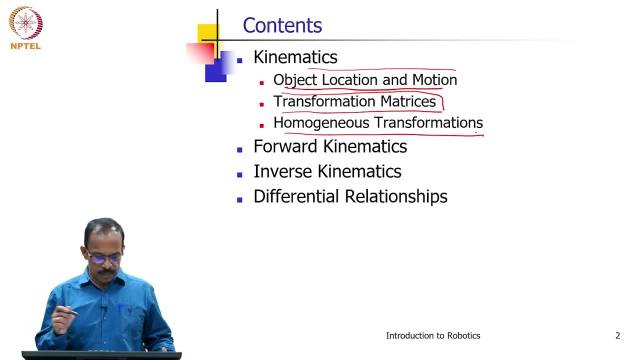 transformation, we need to use something called homogeneous transformations, and once we learn this, then we will talk about the forward kinematics of the industrial manipulators, and then we go to the inverse kinematics and differential relationships. So these are the topics that will be covered in this lecture. So thank you. 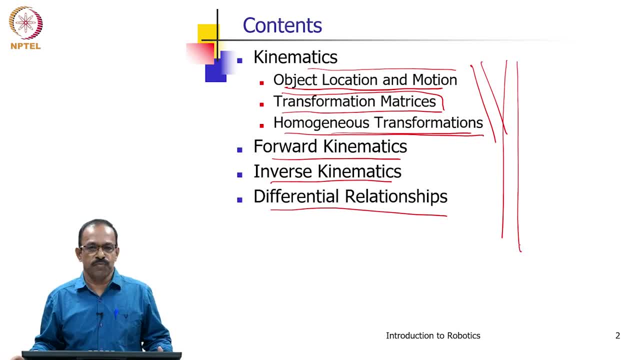 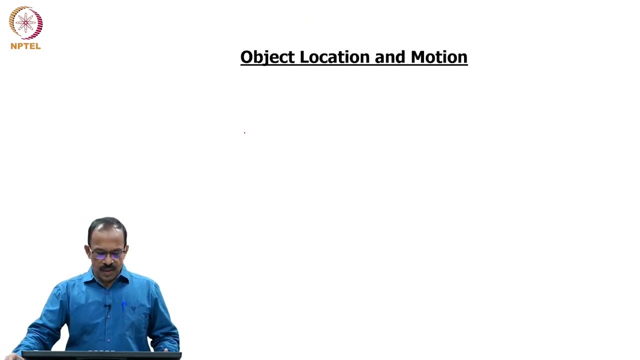 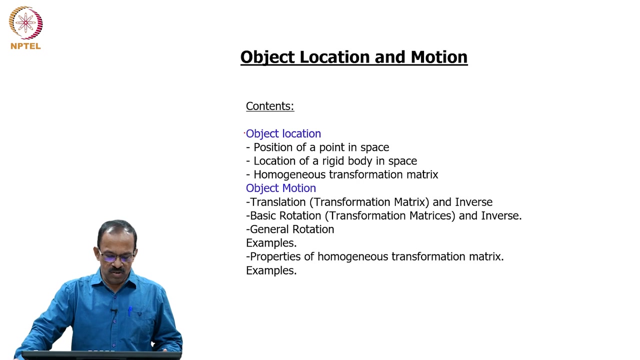 Thank you very much. part of kinematics. So first we will start with the basic relationships of object location and motion. So now, if you look at the object location and motion as the first topic, we can actually see that there are few things we need to understand before we talk about the motion of an object. 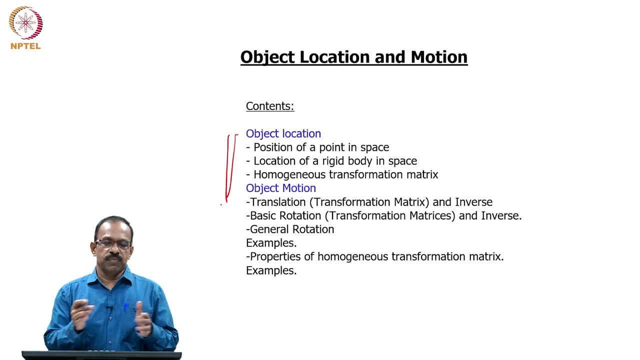 in 3D space. Since you are from different backgrounds- some of you are from civil engineering, some from electrical, some from mechanical, some from chemical- I want to go through some basic mathematical relationships, which some of you may be already familiar. but this is 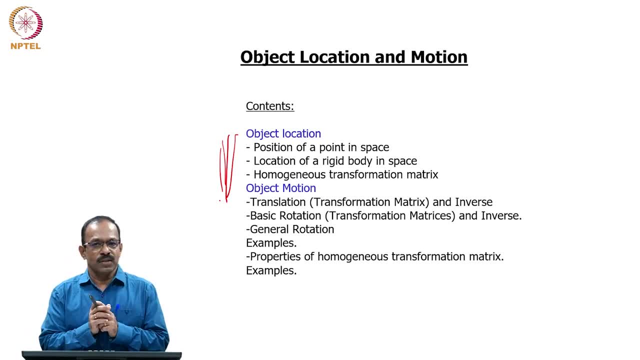 to make sure that all of you understand the basic concepts so that when we go to the forward kinematics and inverse kinematics, you may you will find it easy to follow. So let us start. So the first thing that we will be discussing is the position of a point in space. How do 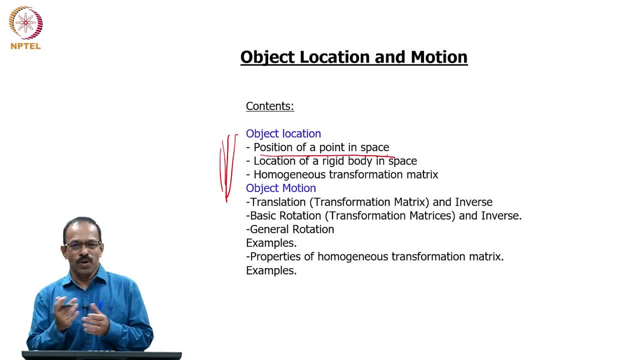 we represent a position of point in space, Very basic thing, which most of you already know. but then we start with that and then see how do we represent the location of a rigid body in space? Because a position of a point in space can be represented, but an 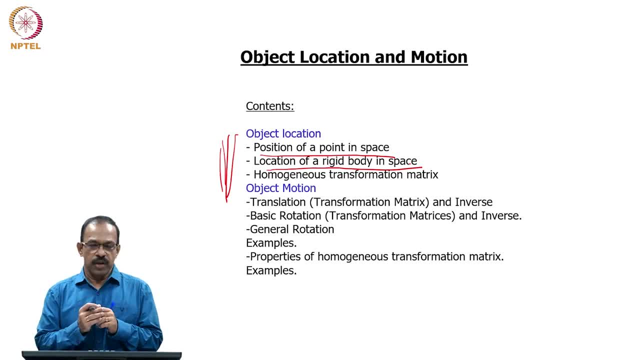 object. when you have an object, it is not only the position you need to have, need its orientation also, because an object, it is a three dimensional object. So a position alone is not sufficient to represent an object, So we need to have the 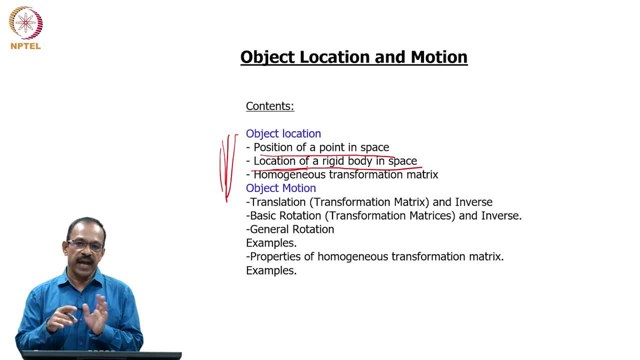 location of an object, where location, says, means the position and orientation of an object. and then we talk about the homogeneous transformation matrix And in object motion we need to see. I mean there are two ways that an object can actually move. So one is the translation. 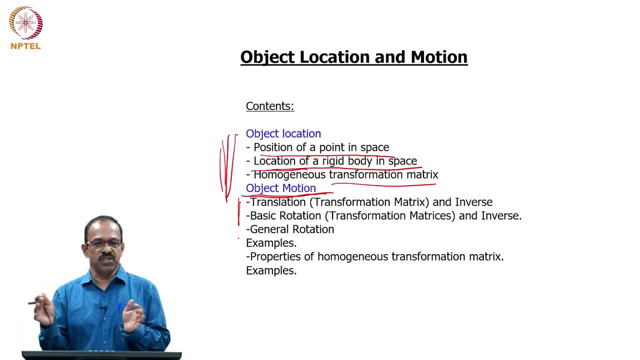 you can actually move linearly from one point to the other point: translation motion, the other one is a rotation, rotary motion. So let us learn the Hollywood method of rotation, rotary motion, So you can have a translation and rotation for an object. So how do we actually 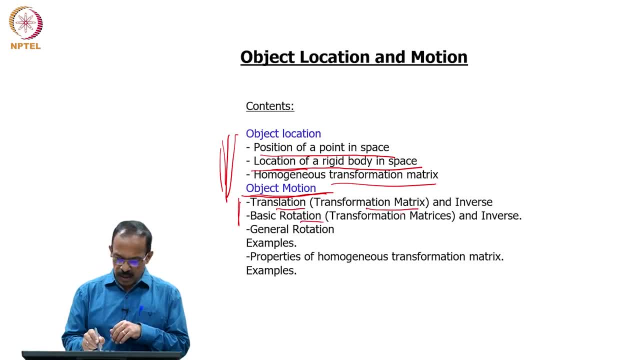 represent this translation and rotation using matrices. that is basically the transformation matrices: translation matrix and rotation matrix- and then we talk about the general rotation principle also, And finally we will have a homogeneous transformation matrix. and then we take few examples to explain how the homogeneous Subs, Representatives, Metrics, can be represented. 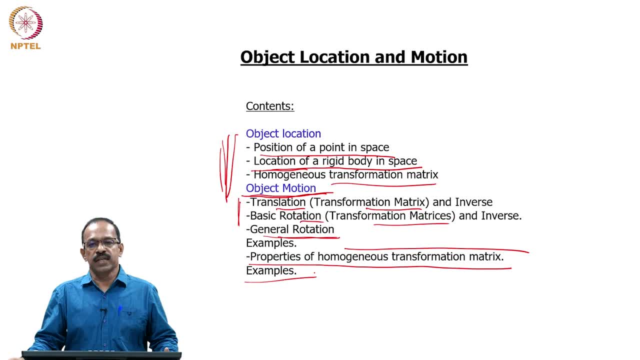 can be used to represent the motion of an object in 3D space. So that is what we are going to discuss in the the first part of object location and motion. before we get into the the robot kinematics far, we first talk about the general object location and motion. 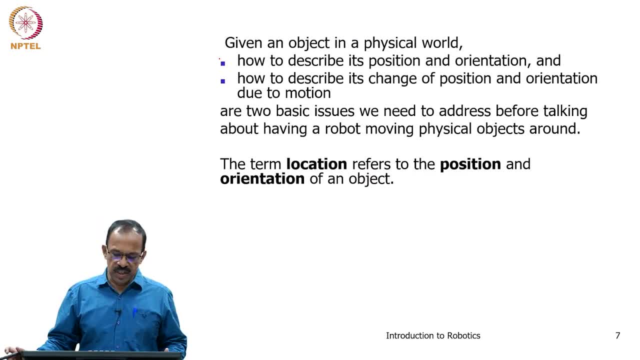 So let us see these. So you have an object in physical world. suppose you have an object in physical world, It is a three-dimensional object, And then it has got some CG and we just put a point there also. Now, if I want to say that, what is the position of this object, or how do you actually represent? 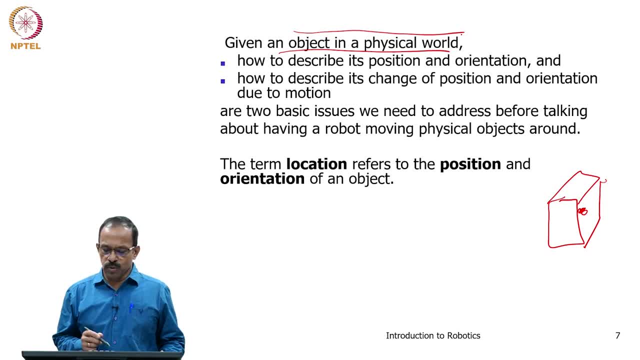 this object in a physical world. So we need to have two things to represent it. One is that we need to know what is the position, What is the position of this object, And then we need to know what is the orientation, because the object can actually be in this. 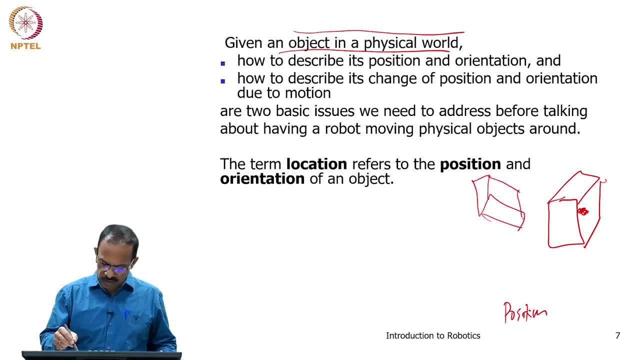 like this way also. we can actually put this object in this way: both are the same object, but the position. if it is the same position, if you actually place it in this orientation, it becomes a different way of representation. So how do we actually represent the position and orientation of an object? and that is basically. 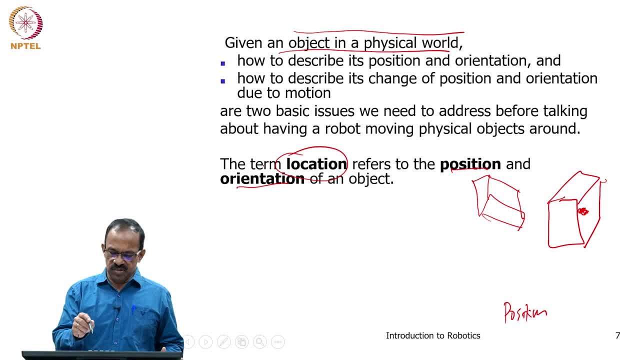 the location of an object And how to describe its change of position also. Now this object has moved from here. This object has moved from here, So this was the initial position. It has moved to here. Now, how do we actually represent this change of position and change of orientation? 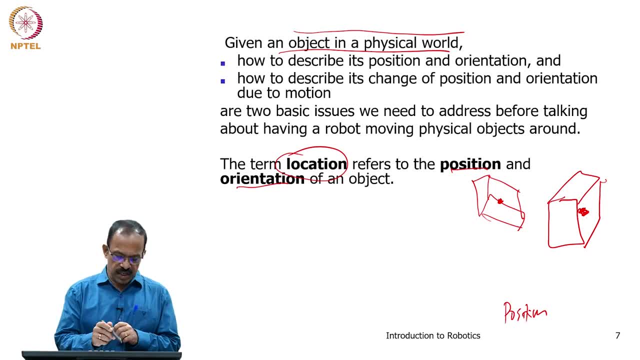 What way we can actually represent it mathematically is the question. That is where we try to see: how do we actually represent this object location in 3D space and when it is moving from one position- Okay location- to another location, how do you represent the this transformation of location? also, 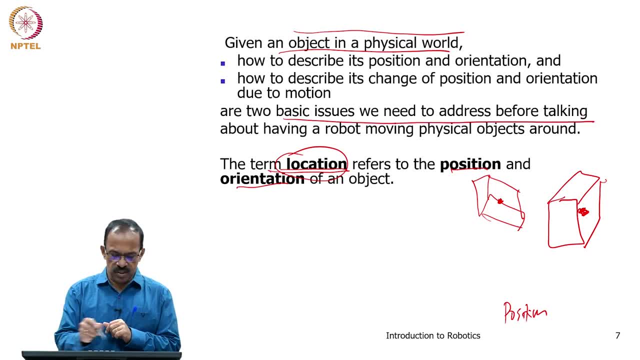 So that is the. these are the two basic issues we need to address before talking about having a robot moving a physical object, because, finally, a robot is being used to move physical objects, So I have an object here. I want this to be moved to here in a different orientation. 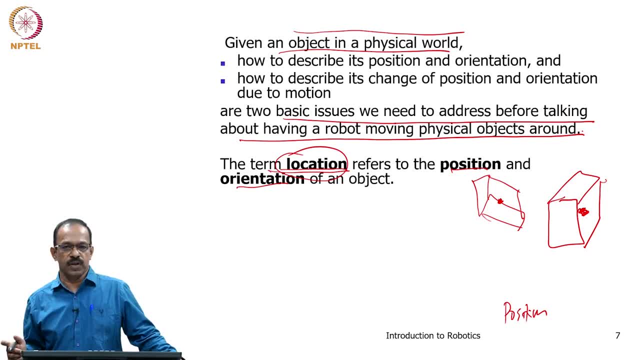 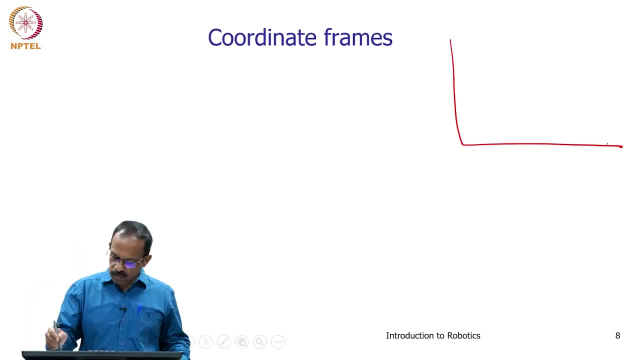 So how do I represent this using in the case of a robot? that can be understood only if we know how to represent 3D objects. in 3D, I mean objects in 3D space. So what we do is to we will try to look at something called coordinate frames using 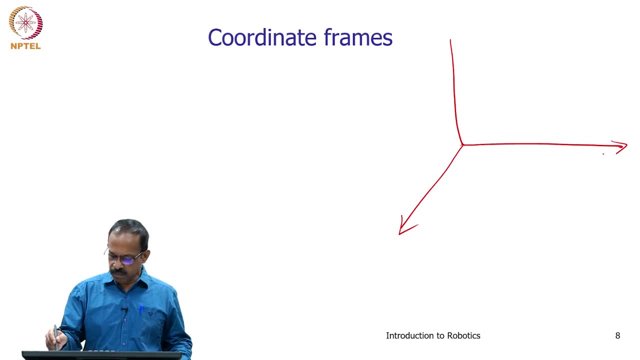 the coordinates of the point. Suppose you have a three-dimensional coordinate frame like this, where we write this as x, y and z. Now we know that if you have a point in space, if you have a point in space, I can actually. 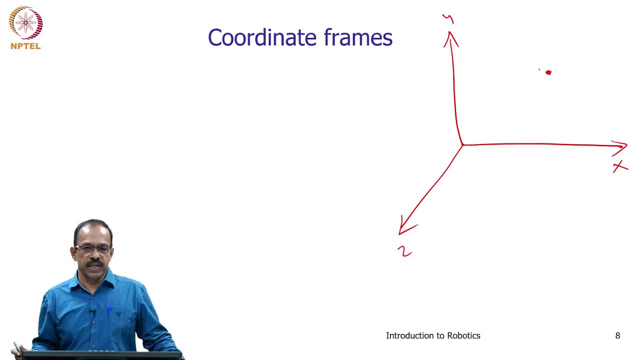 represent this point, So using its coordinates. so I can say that, okay, the coordinates are x, y and z, And then we will say, oh, this is the x coordinate, this is the y coordinate, and this may be the x- z coordinates. so x, y and z. 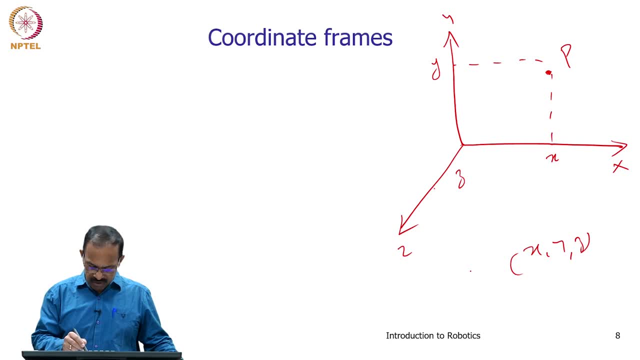 So we will say that this point P can be represented as x, y, z. that is the way how you represent a point in 3D space. this is a vector P. using the coordinate frame, you will be able to represent the vector P. 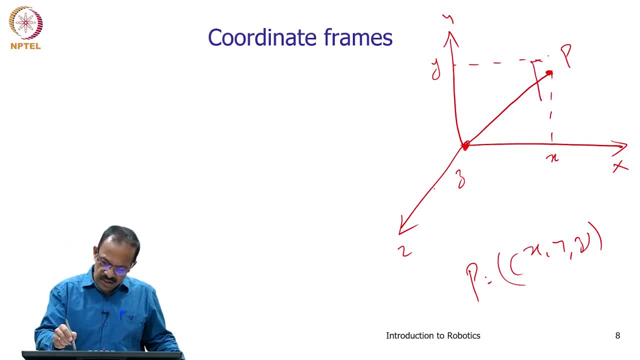 Now, if it is the same as an object in space- suppose this is an object, a 3D object in space- then we can actually say that the position of the center of this object can be represented again using the coordinate points. So you have these coordinates to represent the center of this object. 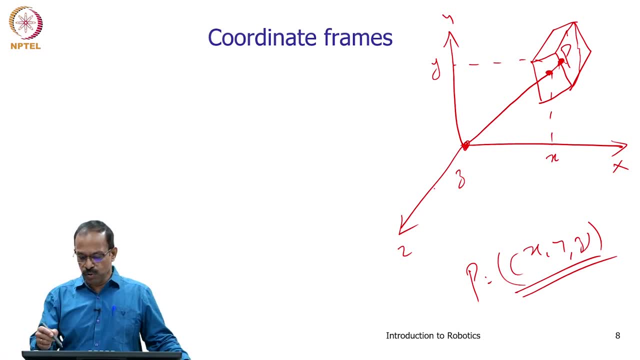 But that is not sufficient in the case of a 3D object, because that actually gives you only the position of the object, But we need to know how this object is oriented with respect to a frame, So we need to always have a reference frame. so we call this as the reference frame with. 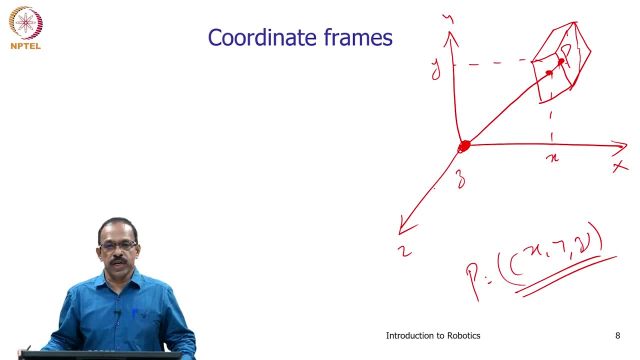 respect to which we can represent a position. So, whether it is a point or an object, we can use a reference frame to represent the position of an object, or a point or an object, And that is what we call it as the coordinate frame. 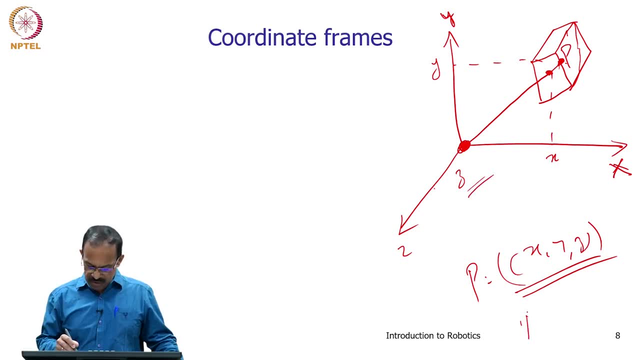 Okay, So this coordinate frame becomes the reference frame to represent the position of an object or a point in 3D in space. so it can be 3D space or any dimensional space. we can use a coordinate frame to represent position of object or a point in the space. 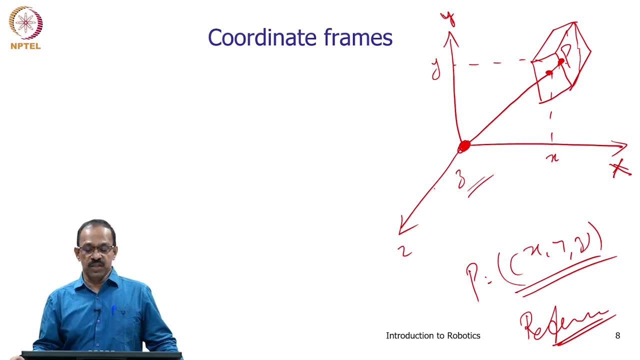 Now, if you want to represent the orientation of the object in space, then we need to have something called. we need to have another reference frame. We will say that, okay, this also has got a reference frame, so we have a frame attached. 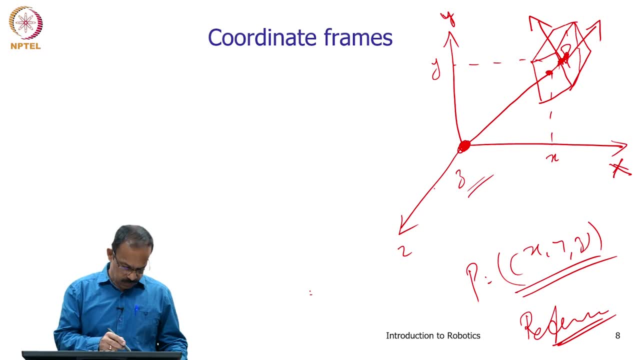 to this which is like this: okay, so I will say that, okay, there is a reference, there is a frame attached to this. so I will say: this is x dash, y dash and z dash. So I will say, okay, this is the frame which is attached to the body. so now we have a. 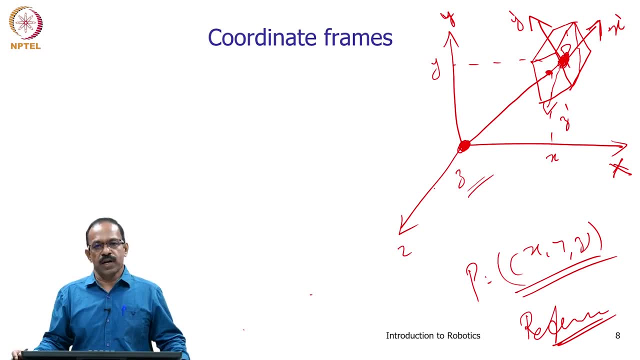 reference frame. Okay, We have a frame attached to the body also. Now the position of the body or this object can be represented as the position of the coordinate frame, this frame. So we, if we know the origin of this frame, then we can represent the origin of this frame. 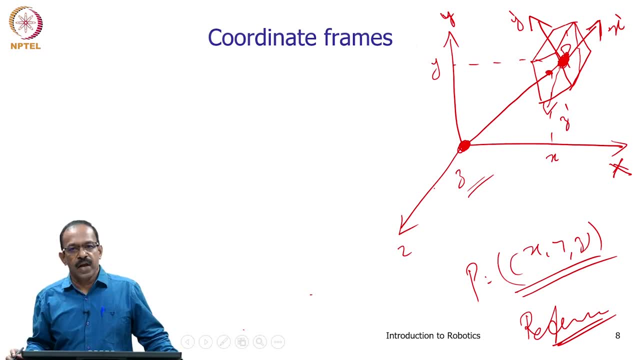 using the coordinates as the position of the object And the orientation of the object can be represented as a as reference to this frame. So what is the orientation of this frame? Okay, So where there is a coordinate frame with respect to this frame, so I call this as the. 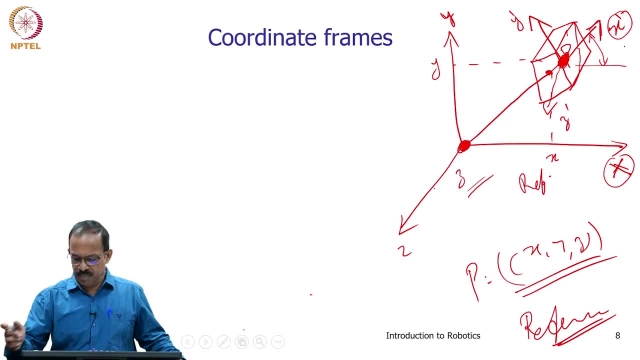 reference frame and I call this as the mobile frame. so I call this as a mobile frame or an object frame, whatever name you want to call. So if I call this is a mobile frame and this is as a reference frame, then I can represent. 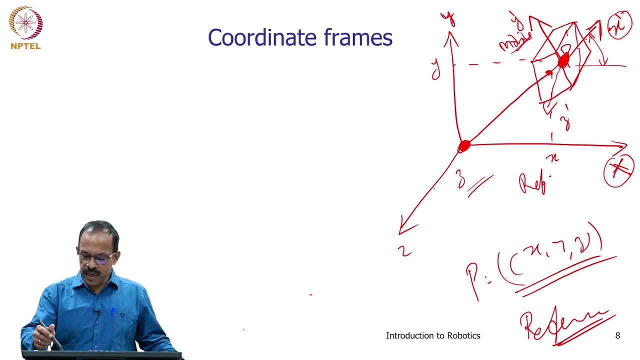 the orientation of the object by looking at the orientation of this coordinate frame with respect to this coordinate frame, so how these two coordinate frames are aligned. that actually represents the orientation of the object. Okay, Thank you All. right now let us continue. 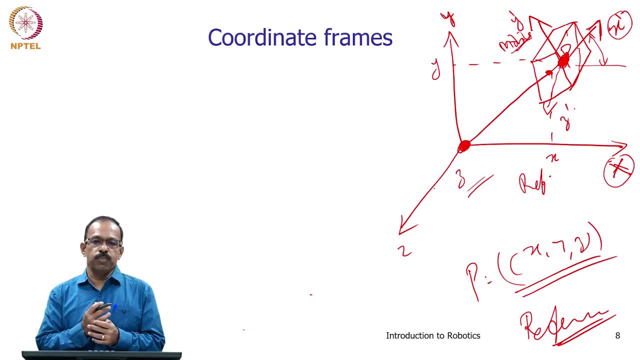 Okay, Well, let us immediately go and write down the container and a model within it as well. All right, the object. So, in order to represent the position and orientation of object in 3D space, we need to refer the. we need to represent them in terms of coordinate frame. 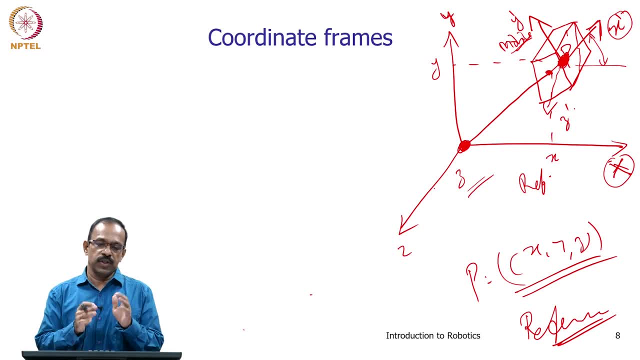 So we need to identify the reference frames and with respect to that frame, we can actually represent the position and we can have a frame attached to the object and the orientation of that frame with respect to the reference frame gives the orientation of the object with respect to the reference frame. 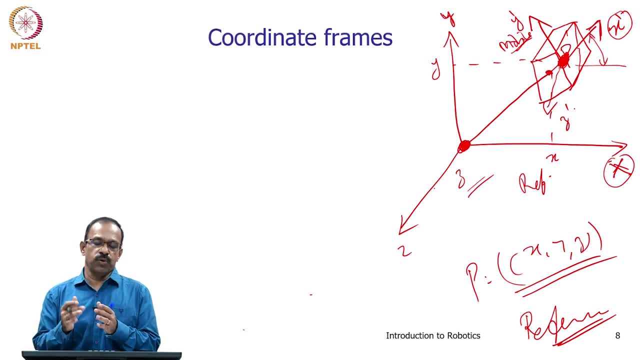 So this way, we can define the position and orientation of objects with respect to coordinate frames. Now, the frame which is used as a reference is normally referred to as a fixed frame, and the frame which is attached to the body is known as a mobile frame. 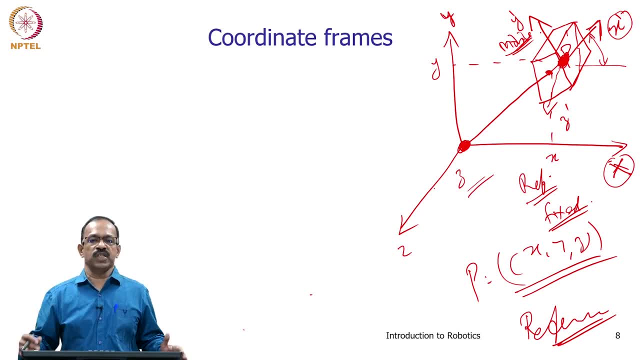 So we have a fixed coordinate frame with respect to which the position can be defined, and we have a mobile frame with respect to the orientation of the mobile frame with respect to the position, So the fixed frame can be used to represent the orientation of the object. 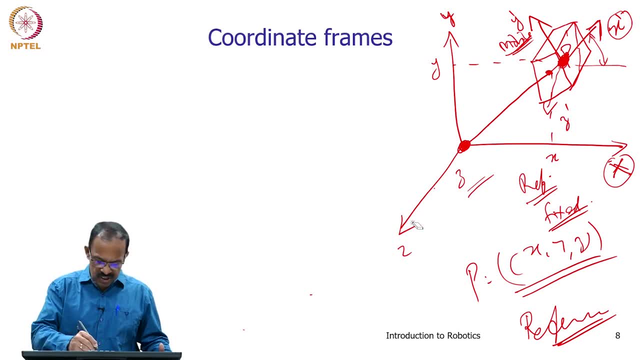 So that is the way how we can represent the position and orientation of objects in space. Now let us see, let us go to the basic definition for the coordinates, coordinates and the coordinate frames, and then see how we can represent the orientation using the coordinate frames. 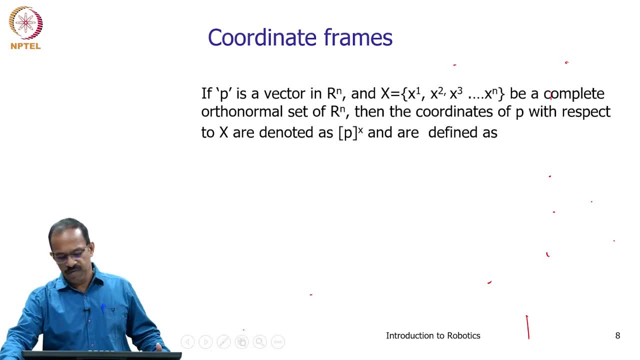 So now, if you have a vector p, So you have p factor. Now p is a vector in r-dimensional space, I mean n-dimensional space, where r is Rn is the n-dimensional space, then the coordinates of p with respect to x are denoted as px. 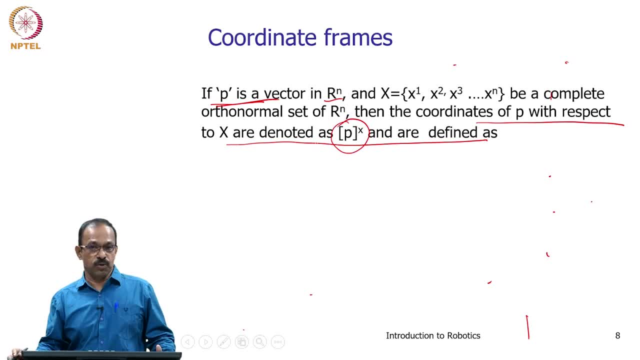 so the coordinate of p with respect to x are denoted as x and the vector p can be defined as sigma. k is equal to 1 to n, px, k, x, k. so this is the way how we can actually define the vector. 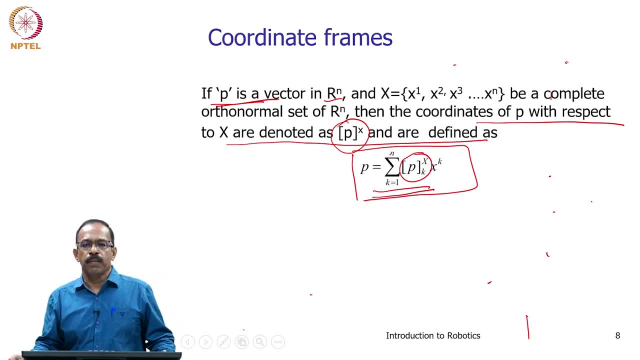 So if you have a vector p, that vector p is a vector. So as long as p, whether it is where this is the coordinate of P with respect to the kth axis. So we have the x1,, x2,, x3,. 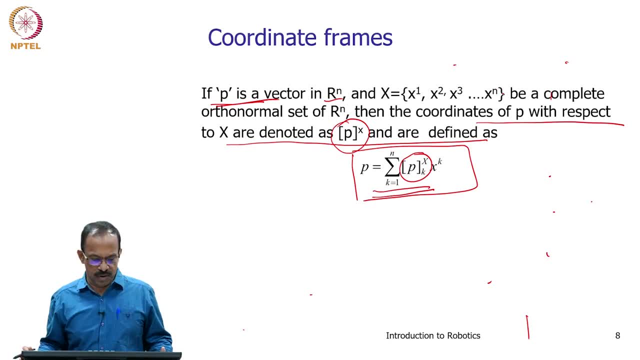 xn as the axis of the coordinate frame or the n-dimensional coordinate frame, Then we will get this as the coordinates of P with respect to x and Px. xk is the complete vector. how you define the vector in n-dimensional space? Now it is a 3-dimensional space. we 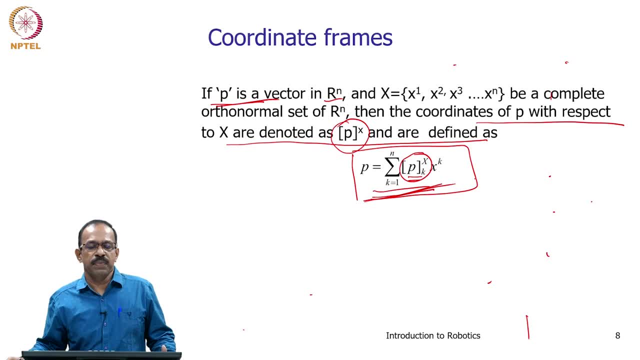 will be able to see, that is, P1, P2, P3 will be the coordinates and we will be able to get the vector. Now how do we actually define this coordinate? Suppose you have a coordinate frame like this and this is your P, then this is the coordinate. 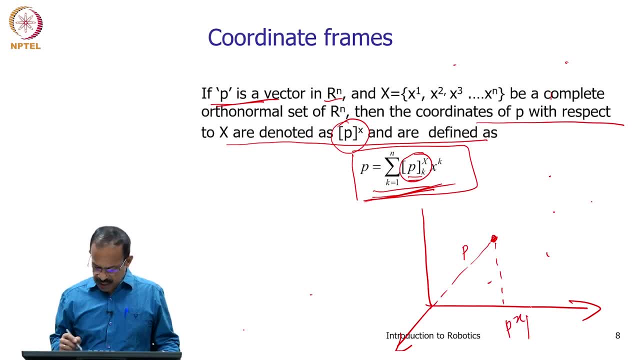 of your Px, that is the coordinates of P in the x axis. So that is the Px. Now, this Px can actually be obtained as by taking this vector P. So if you take the dot product of P with respect to x, then we get this as Px, that is the dot product of this vector. 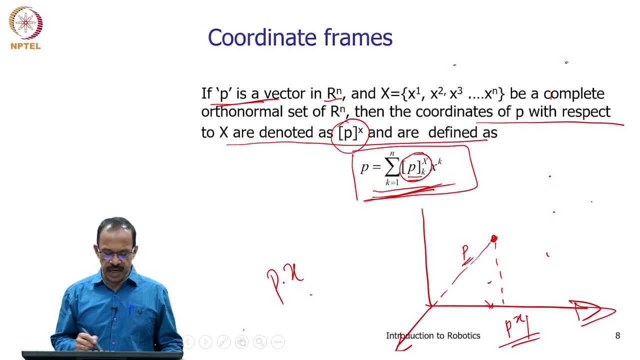 with the unit vector of x axis, you will be getting this as Px. So Px, or the coordinate of P with respect to x, is nothing but the coordinates- Yes, dot product of the vector P with respect to the x axis. Similarly, P- y will be dot product. 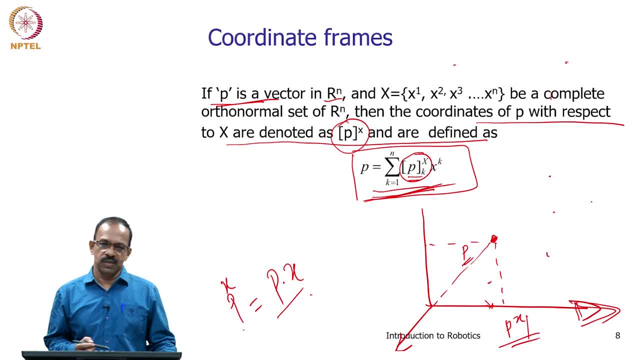 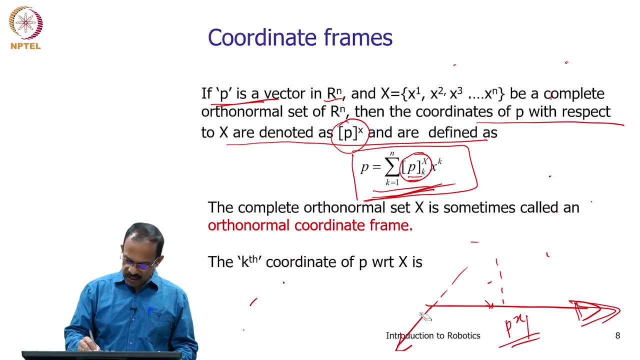 with respect to y and P z will be dot product with respect to z. So that is the way how we actually define the coordinates of P in this coordinate frame. So the kth coordinates of P with respect to x is defined as P dot, x, k. So we can see. 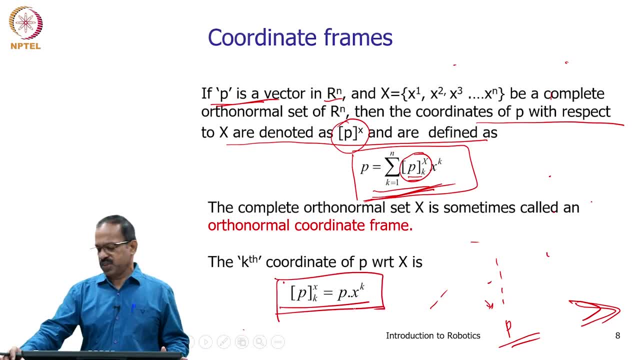 that the kth coordinate of P with respect to x or with respect to the coordinate frame x, is x1, x2, x3, depending on the number of the dimension of the coordinate frame. So here, if it is in the 3 dimensional coordinate frame, then you have: k is equal to 3 maximum. 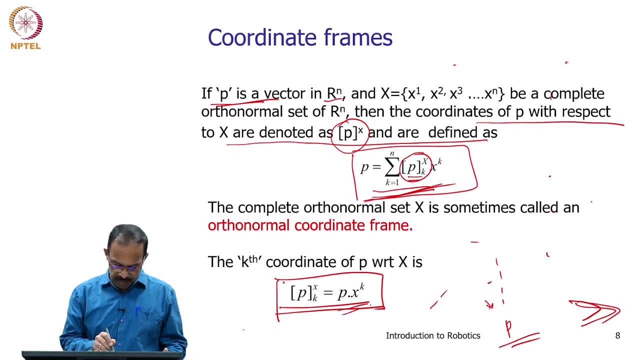 ok, So this is P x k. is P dot x k. So if it is P with respect to x, then we have this coordinate: p x k as p dot x k. So you take the dot product of the vector p with respect to the kth axis, you will get the coordinate of p. So this: 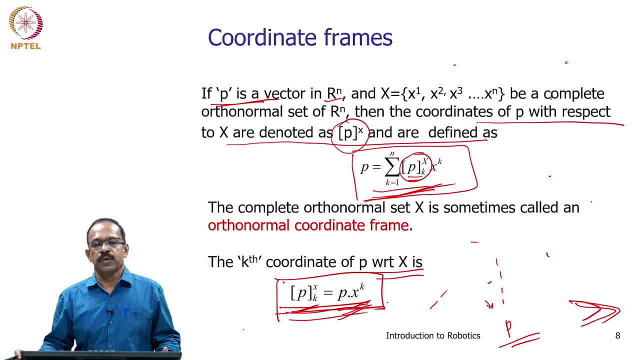 is the way how we define the coordinate of a point in space. Now, if you have, that is the explanation here given here. so you have this as p 1 x, p 2 x, etcetera. So you have this as this is the p, that is the vector p, and p 1 x is nothing. 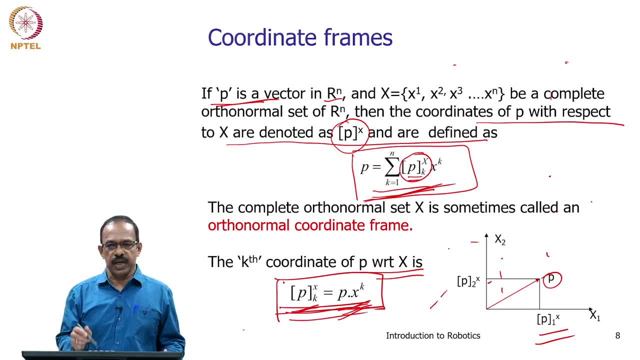 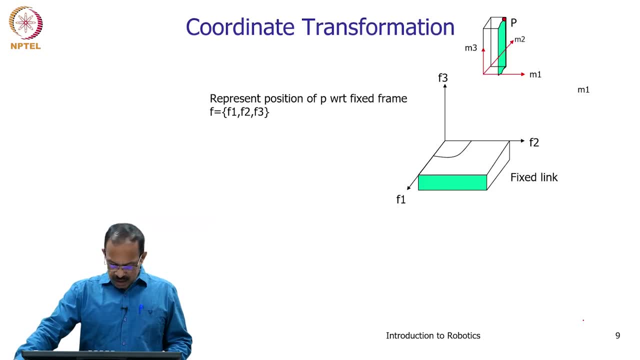 but p dot x 1 and p 2 x is nothing but p dot x 2.. So that is the way how we get the coordinates of p. Now having Now, having seen this, now we need to look at how do we actually represent this in different situations. 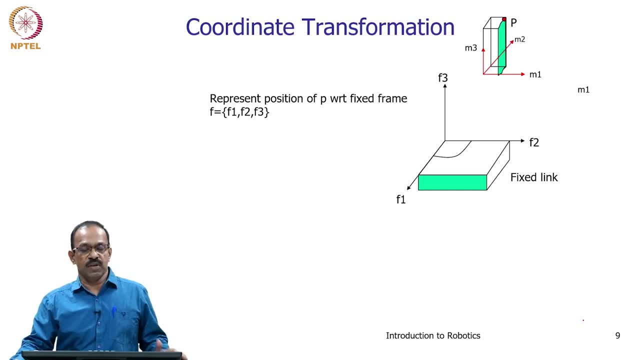 that is, how do we actually represent the transformation of an object? that was about the point p. Now suppose we have an object like this. suppose we have an object three-dimensional object. In the three-dimensional object we define the coordinate frame as m 1, m 2, m 3.. So 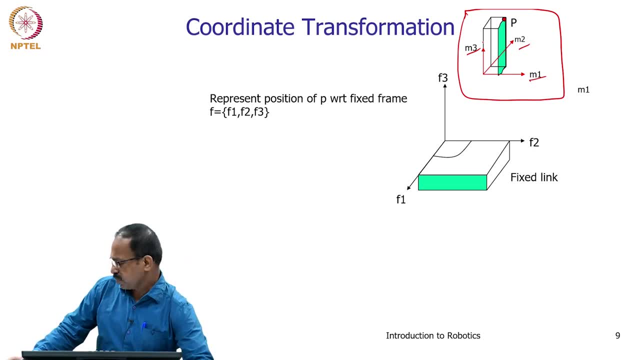 we define a coordinate frame: m 1, m 2, m 3.. So we define a coordinate frame: m 1, m 2, m 3.. Suppose this is. I take this as an object. so I have a object, three-dimensional object. 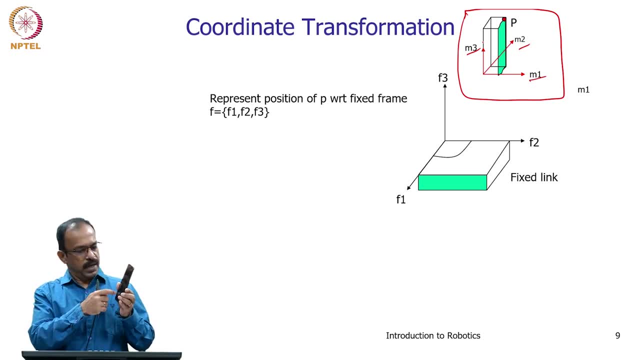 and I define a coordinate frame like this: m 1,, m 2, and m 3, three-dimensional coordinate frame And, as you can see, I define a point p at one corner. so I can see I can define a point p like this in this coordinate frame. 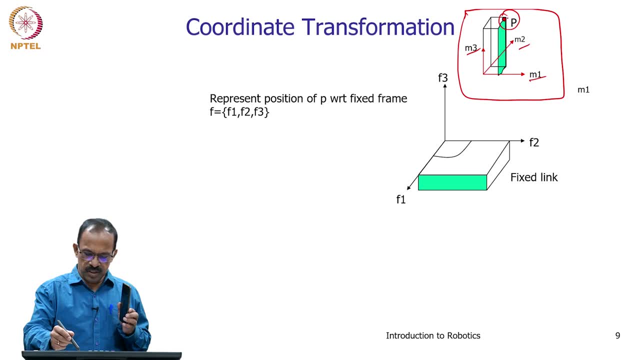 So, as you can see, I am using these points and this is the origin of the coordinate frame, and m1, m2, m3 are the axis of this coordinate frame. Now this point P, so the coordinates of P can actually be obtained by taking P, dot, m1,. 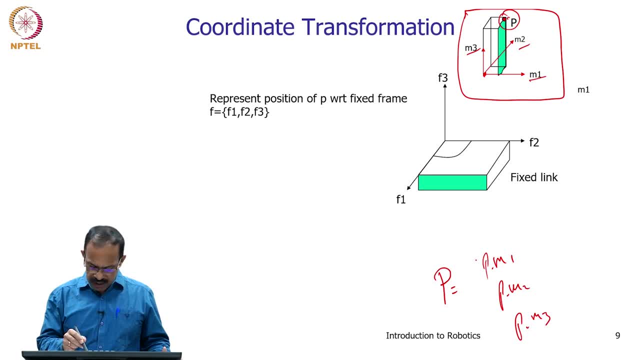 P dot m2 and P dot m3.. So that will be the coordinates of P with respect to the frame m1, m2, m3.. So I attach this to the object and therefore I call this as mobile frame. I assume that. 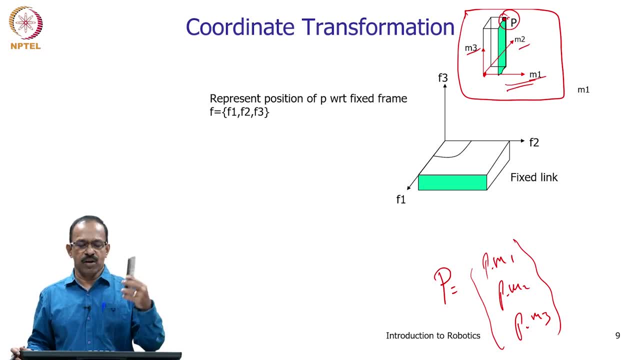 it actually moves along with the object. the frame moves along with the object, so I call it as mobile frame And I will be defining this. I mean the point P here and I will get the coordinates as P dot m1, P dot m2, P dot m3. 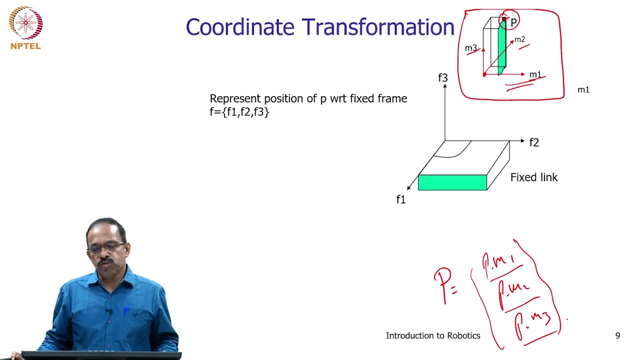 Now let us see what happens. Now I assume that this object is rotating by 90 degree or 180 degree. So I am having this object and this point is P. I am assuming that it actually rotates by 180 degree, so it actually move like this and the point is P. now here: 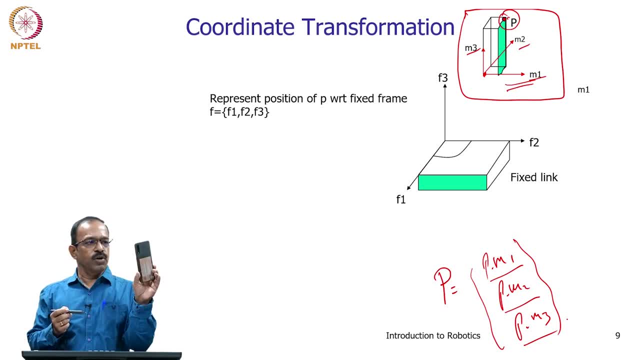 So point P has- I mean it has- rotated, and I want to know what is the position of P after the, after rotation. So the object has rotated 180 degree And I want to know what is the rotation of the object. So I want to know what is the position of P with respect to the frame. now, 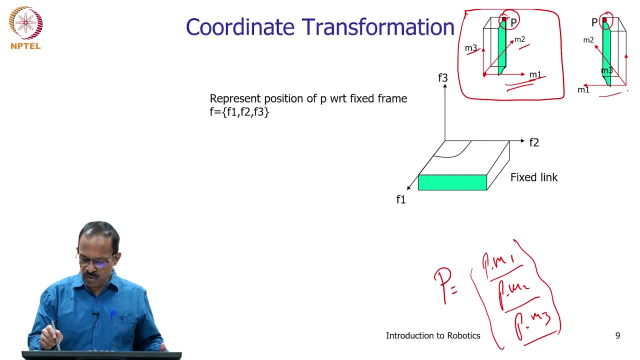 So now the P is this and you have this frame also rotated, like this. I mean, along with the object, the frame rotated, and you want to know the position of P. So what will be the position of P now? will it be the same as previous one, or the P will? 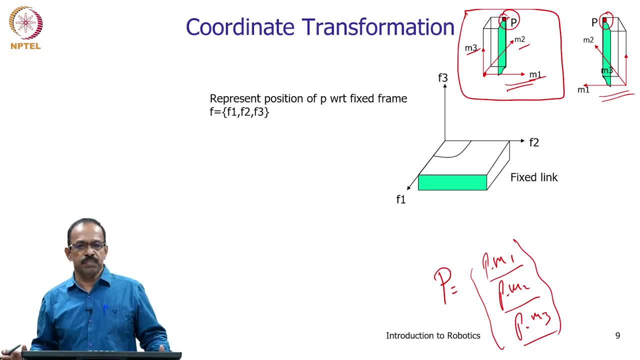 change. now the position of P will change with respect to the frame, so it is not going to change, Because now P will be again. P is P dot M1, P dot M2 and P dot M3, so that is the coordinate. 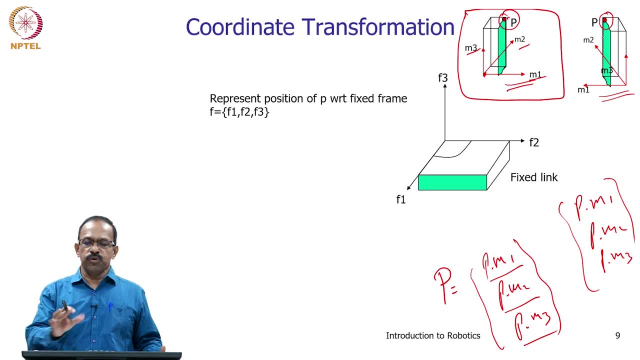 of P and since M1, M2, M3 also rotated along with the object, there will not be any change in this coordinates of P. so P will remain same. So any point P in this three-dimensional object will remain as the same as the object moves. 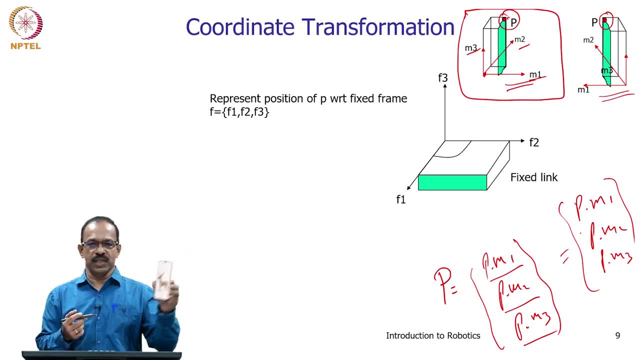 object. So P rotates or translates whatever it is, because the coordinate frame also moves along with that. therefore, the coordinates of P remains same as it as the object moves. So there is no change in the position of P with respect to the mobile frame. 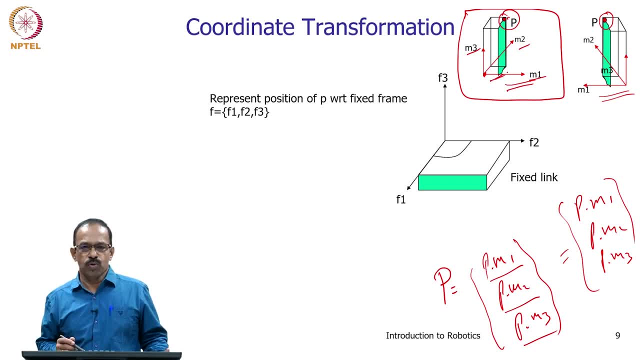 Now assume that this object, we actually move this object to or we actually place the objects in this frame. I have a fixed frame now. so I have a fixed frame. I will say that the fixed frame is this one. I will assume that there is a fixed frame with respect to my body or the room. I will 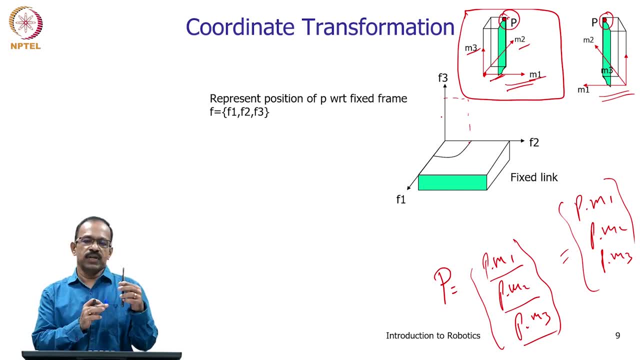 say that I am initially aligning this object with the fixed frame such that the axis of mobile frame and the fixed frame are aligned. that is, I am placing it like this. I am placing this object in this frame with a fixed frame. There is a fixed link, or I have called this as fixed frame: f1,, f2,, f3. 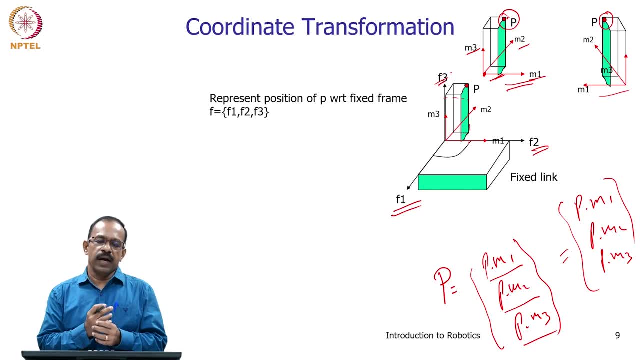 So f1,, f2, f3 is a fixed reference frame and initially I place this object P in the in this frame, aligning M1 with the. it is slightly different in this case, but assume that it is: M1, M2, M3 are aligned in this case. 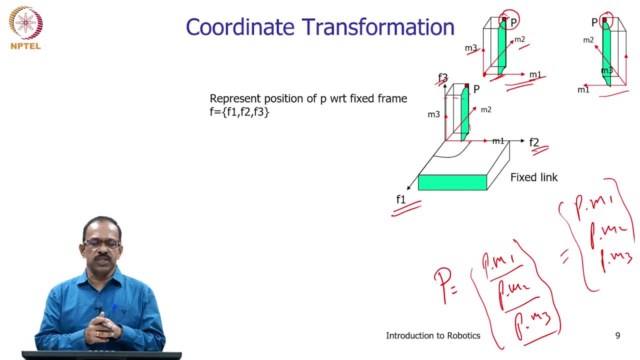 Now, if I align this and then get the points, P with respect to M will remain the same. Okay. So P with respect to M will remain the same here. Now I will find out what is the point of P with respect to F. So I am interested in. 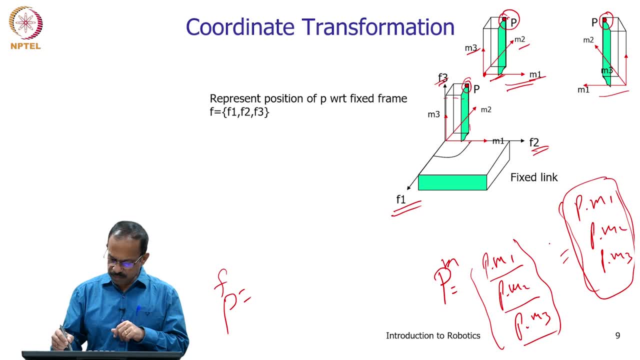 knowing now what is P F. So this was P M mobile frame. I am interested in knowing what is P F. what is the position of P with respect to the fixed frame? I can actually get it again by using the same principle. I take P dot F1, P dot F2 and P. 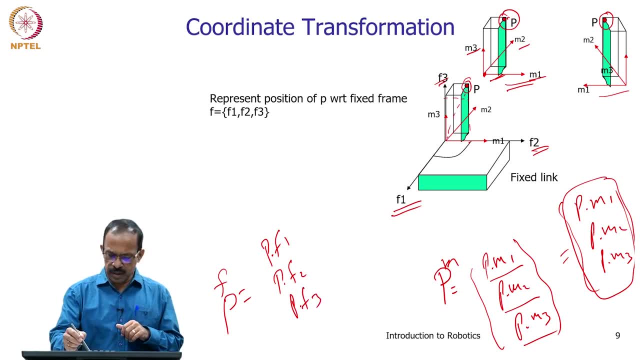 dot F3, I can take the dot product of this vector, P with respect to F1,, F2, F3, I will get the position of this, And the position of P with respect to M will be P dot M1, P dot M2, P dot M3. 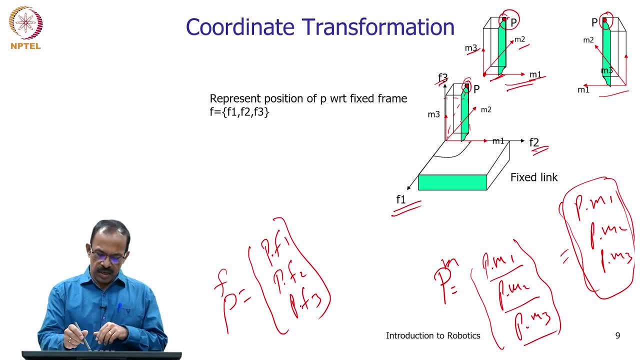 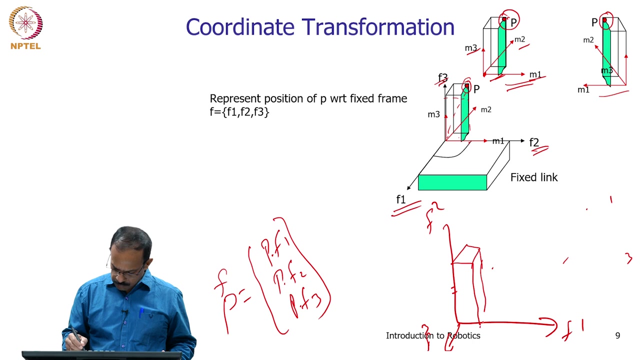 Now, if I rotate this object 90 degree now at this location, if I rotate it by 90 degree, so initially we have this. I put this F1, F2 and F3 and we had this object and we had this M1, M2 and M3, so this was point P. 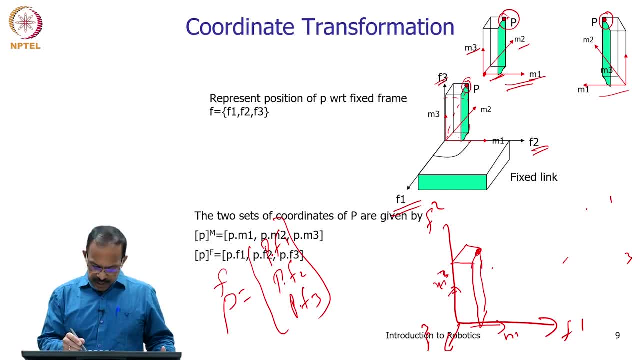 Now, if I have rotated this object by 90 degree and this P, actually, I have turned this and the object actually came like this and the P actually reached here this position. so this is P now. so M1, M2, M3 also rotated. 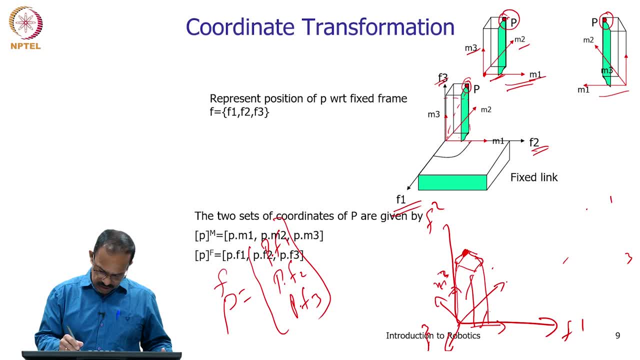 so now M1, M2 and M3 has gone like this: This will be P M1,, this will be M2 and this will be M3.. So you have this object. initially, this object was in this position and it rotated by 90. 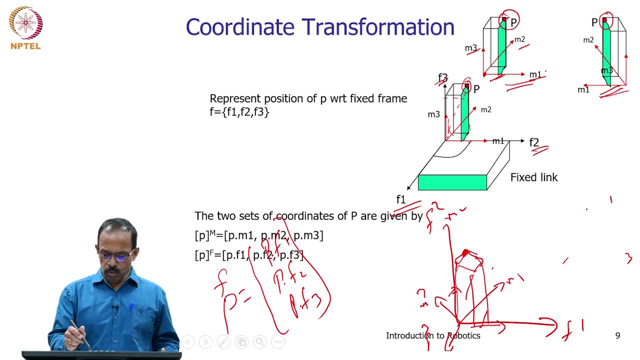 degree or 180 degree, as like this, and the object has actually moved this position and the P has actually reached here. Now, if I want to get the position of P after rotation, so if I get the position of P after rotation, so P with respect to mobile frame after rotation will again remain the same. 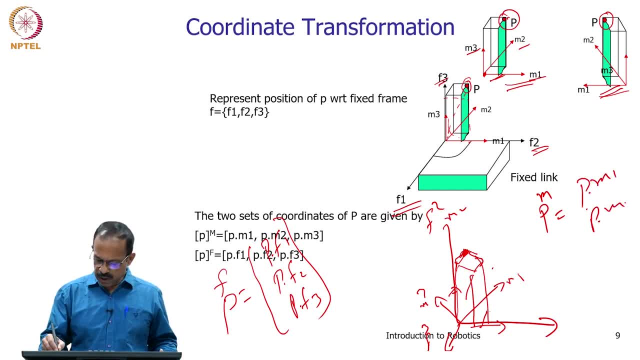 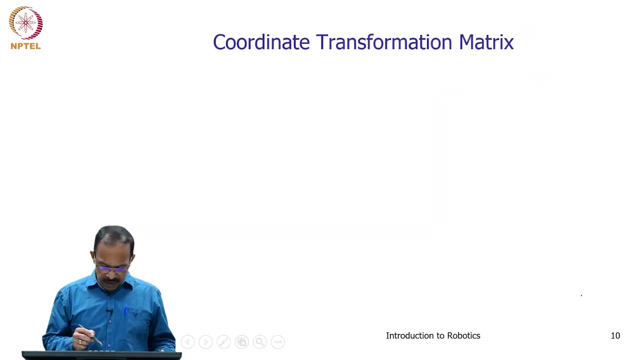 So the rotation will again remain same as P dot M1, P dot M2, P dot M3.. So there is no change in the position of P with respect to mobile frame, But since this is rotated by 90 degree, its position with respect to F can be still represented. 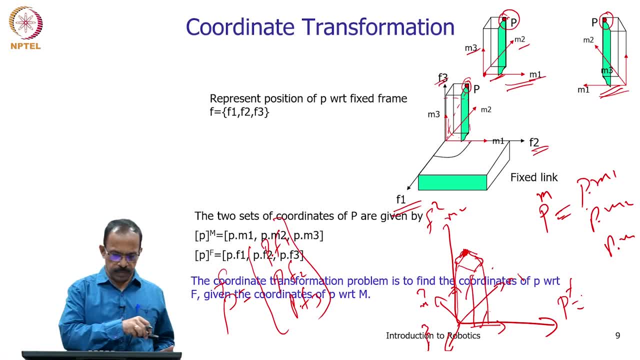 using the P dot F1, P dot F2,. it can be represented using P dot F1, P dot F2, P dot F3, but since, since this object has changed and its mobile frame has moved, therefore the values of P 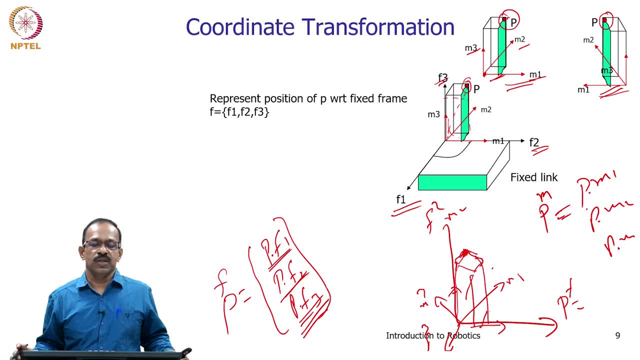 dot F1, P dot F2, P dot F3 will not remain same because the object has rotated. So what I actually say is that when the object is rotating, the position of P remains same with respect to a mobile frame, but its position changes with respect to the fixed frame. 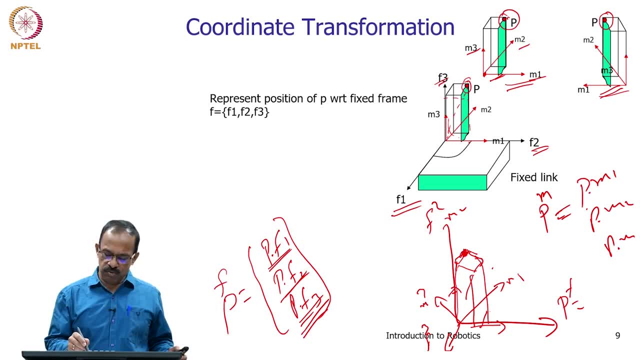 And therefore we need to, if we need to represent the position of P with respect to the fixed frame. Thus the rotation will remain the same- the fixed frame when it is moving. we will need to find a method to find out what is. 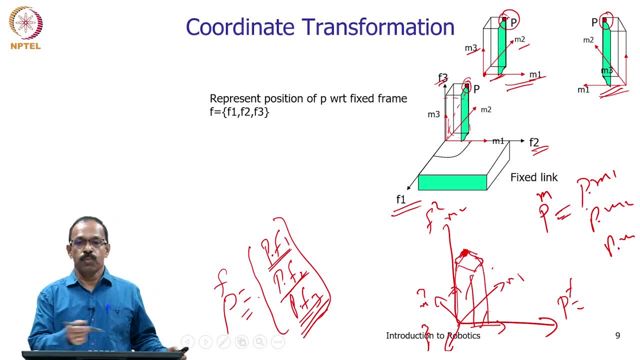 PF when the object is moving with respect to the fixed frame or with respect to its one frame. So that is basically the transformation of coordinates. How do we represent the position of a point in 3D space or position of a point in an object? 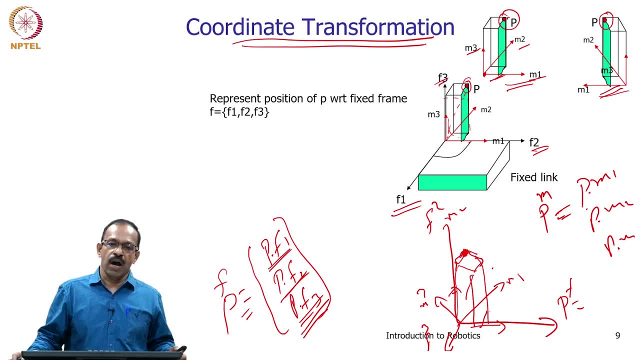 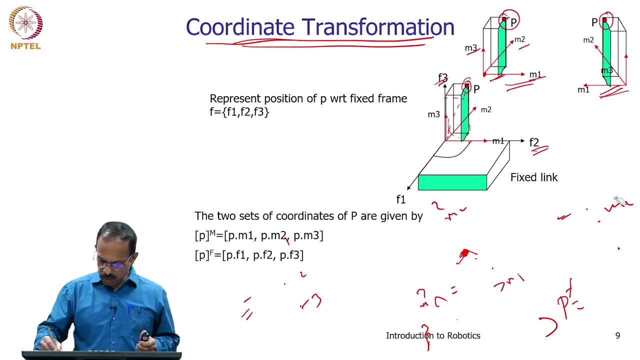 when the object is moving with respect to a reference frame. How do we represent the position? is the question of coordinate transformation. So let us look at this in a slightly detailed way. So assume that the P, the two coordinate frames, PF, PM, is basically P dot, M1, P dot. 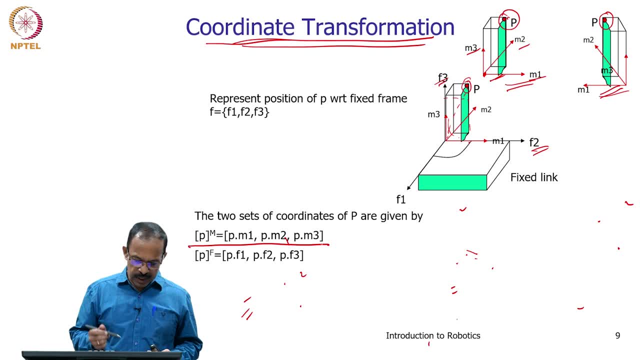 M2, P dot M3, as you can see. So this is P dot M1, P dot M2, P dot M3.. Now, this is P dot F1, P dot F2.. That is the point. P with respect to fixed frame can be represented using P dot F1, P. 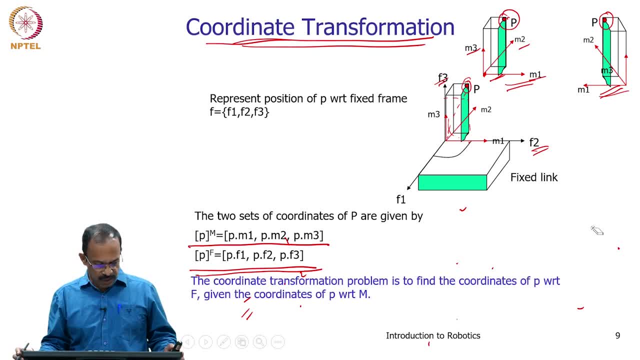 dot F2, P dot F3.. Suppose there is a rotation. so the coordinate transformation problem is to find the coordinates of P with respect to F, given the coordinates of P with respect to M. Suppose we know the coordinates of P with respect to M, how do we find the coordinates? 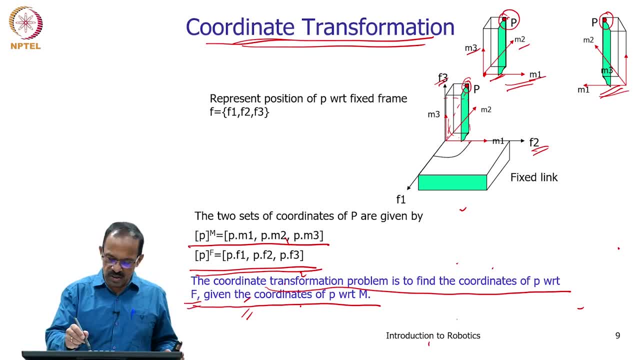 of P with respect to F is the coordinate transformation problem. So we have this P known with respect, known with respect to M, and we want to know what is P with respect to F when this P is moving, when this object is moving? how do we actually represent P with respect to F? 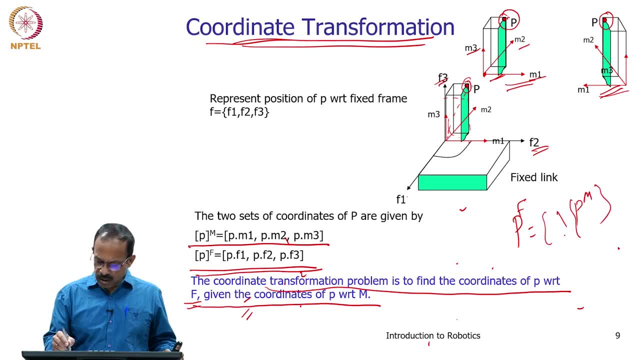 if we know P M and when it is moving, when the object is moving, how do we represent P F if we know P M? because P M remains same. with respect to the mobile frame it remains same, but with respect to the fixed frame it changes because of the motion of the object. 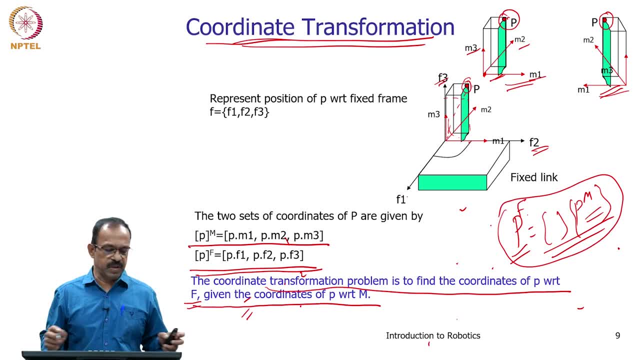 so how do we represent P F if we know P? M is basically known as the coordinate transformation problem. So we know the coordinates of P with respect to M, but we want to know coordinates of P with respect to F. so we want to know this P F when this P is moving. it is moving in. 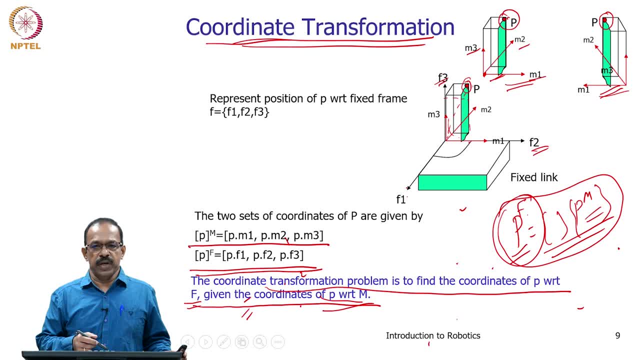 different ways still. we want to know what is the P with respect to F, so that we can represent the Position and orientation of the object with respect to a reference frame. whatever happens to the object, whether the object is moving, rotating, translating, we still want to know. 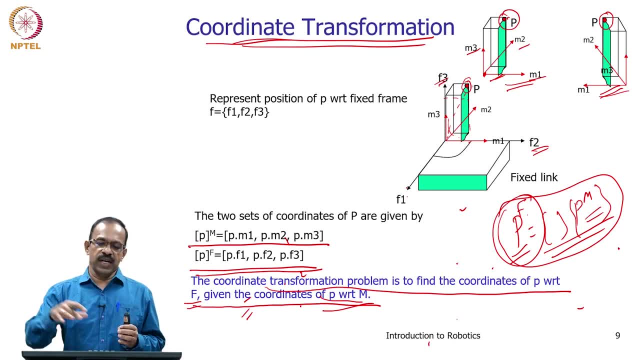 what is the position and orientation of the object? So, if there is a car or a mobile robot in the room and the mobile robot is moving around, so we want to know its position, so we need to have a reference frame and we want to know. 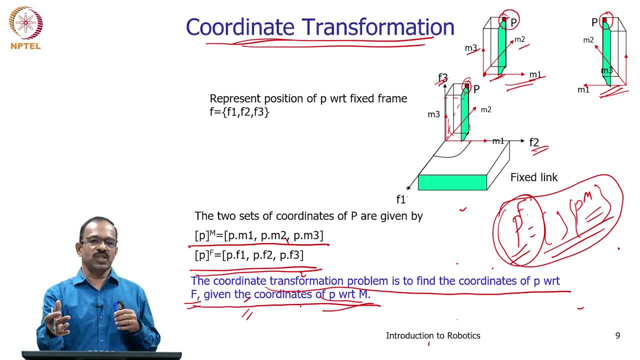 its orientation also. so if you want to know the position and orientation of the robot in the room, we represent the position with respect to a reference frame and the orientation. we will find out the mobile frame and then see how much it has rotated and we will try. 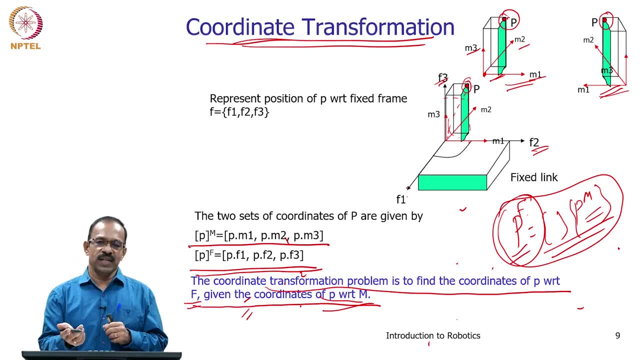 to find out the orientation also. So the question here is: how do we get this P, F, that is, the fixed frame coordinates when there is a movement for the object, and for the point P, which is when it is moving, how do we represent, is basically the coordinate transformation problem. 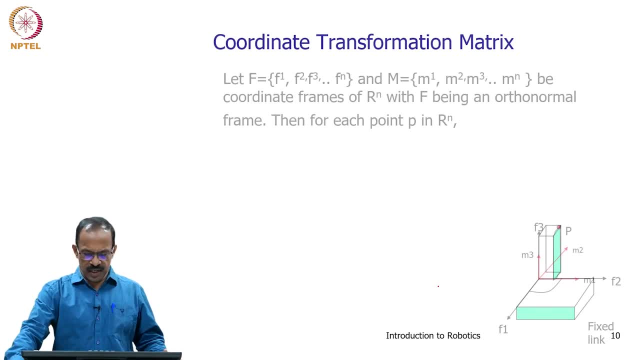 Now, If we look at the Now, If we look at this in detail, we can see that so the F is the frame with F1, F2, F3, and M is the frame with M1, M2, M3 coordinate frames and F being an orthonormal frame, then for 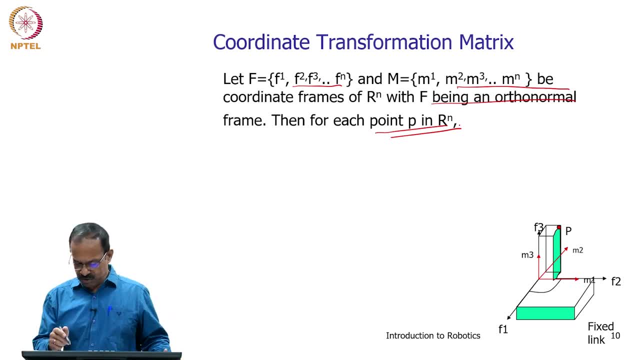 each point P in Rn. that is the point P in Rn. as you can see, this is the point P in Rn. we can say that P F is equal to A P M. So we can represent P F as a matrix A multiplied by P M, and this A is an M by N coordinate. 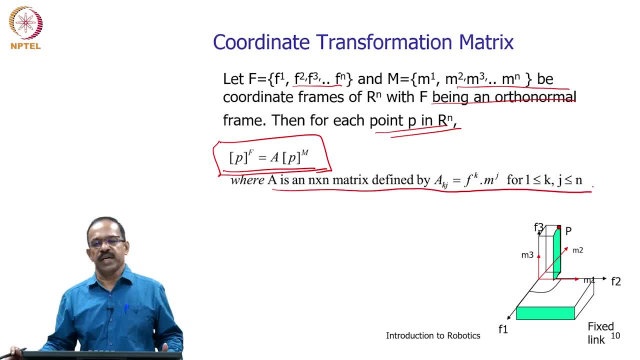 So this A is an M by N matrix defined by FK dot M, J. So this A is known as the coordinate transformation matrix. So basically we are telling that we can write P F as a matrix, A multiplied by P, M, that is. 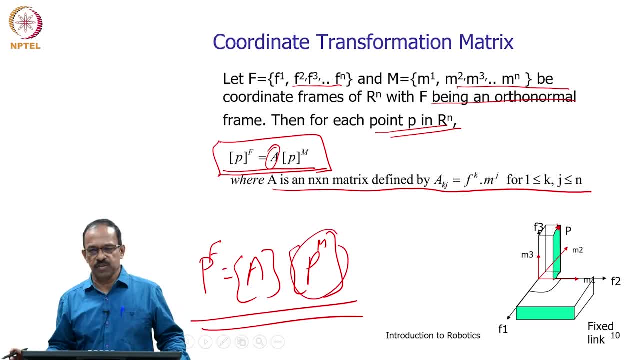 if we know P M, if we know this P M with P with respect to mobile frame, then the point P with respect to the fixed frame can always be represented using this relationship. So this relationship where A multiplied by P M, where A is known as the coordinate transformation, 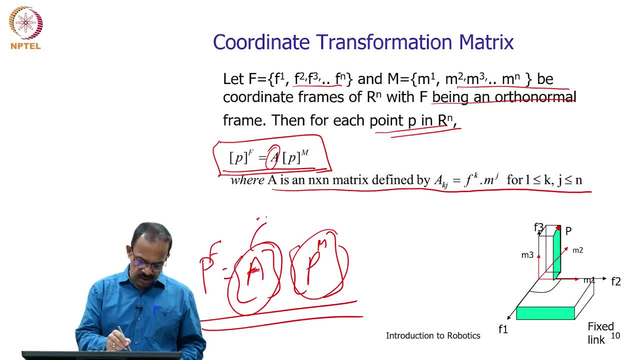 matrix and the elements of this transformation matrix can be obtained as FK dot M J. So F is the fixed frame, M is the mobile frame. F is fixed frame, M is the mobile frame. so FK dot M J gives you the elements of A K or A K J. 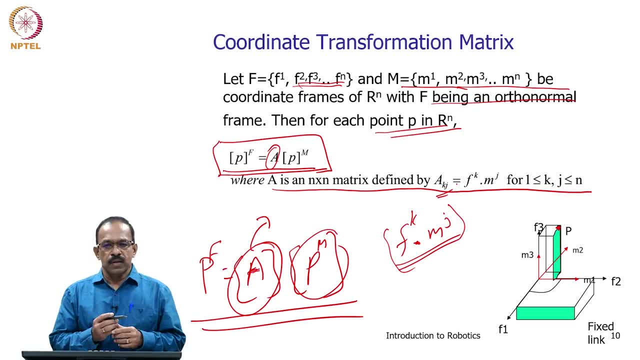 So if it is a three-dimensional frame, so if you have F1, F2, F3 and M1, M2, M3, so you can see this: initially they are aligned, so FK, F and M are aligned, and then, when it is, 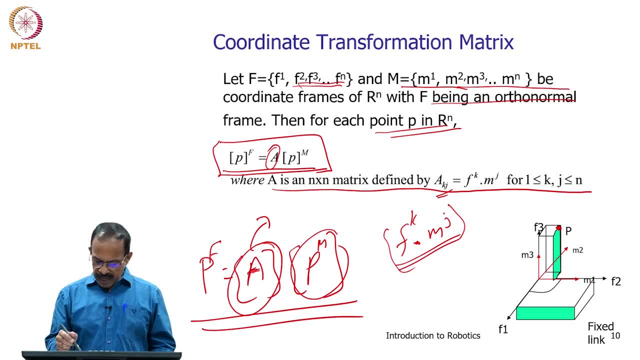 rotating, you will be having a different point to be represented, and that point of that P can be represented with respect to F by using this A. So now, if you write A for a three-dimensional matrix, So for a three-dimensional space, F1, F2, F3, and M1, M2, M3, then we can say that A11. 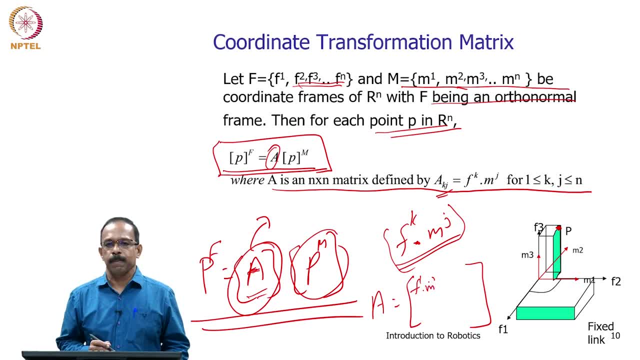 is F1 dot M1, then F1 dot M2 and F1 dot M3, three elements. Similarly F2 dot M1, F2 dot M2 and F2 dot M3.. Similarly here: F3 dot M1, F3 dot M2, F3 dot M3.. So this is the way how you get the transformation. 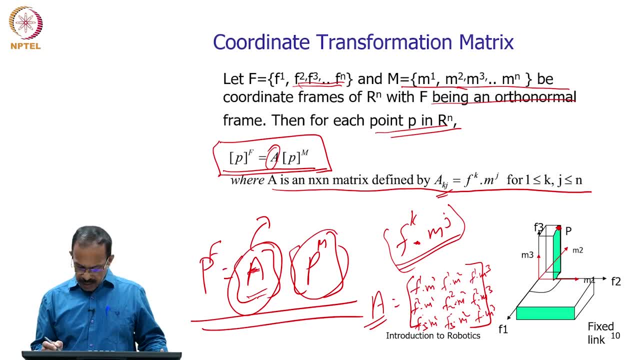 matrix. So basically it says that if you have F1, M1, F2, M2, F3, M3 and if there is a rotation, now these are aligned. so you can see, in this case F1 dot, M1, so this is so. they are not. 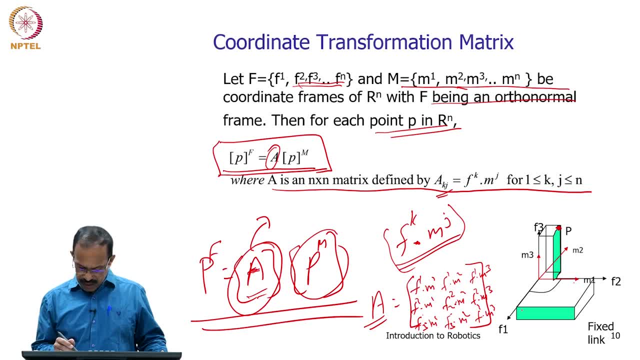 aligned, And this is M1,, this is F1,. so F1 dot M1, will be 0.. Yeah, So there will be. they are not aligned, so you will be getting it as 0.. So, whenever there is an alignment, you will see F3 dot M3,. you will see F3 dot M3 is 1.. 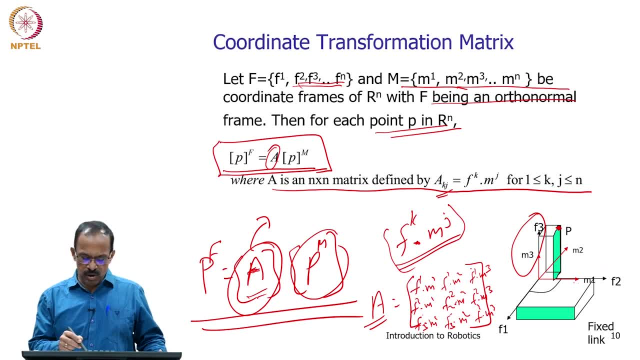 And same way you can get F2 dot M2, F1 dot M2, etcetera, and you will be able to get this matrix A. that is a transformation. matrix A, So the transformation between two coordinates. So these are two coordinate frame: one is mobile and other one is fixed. 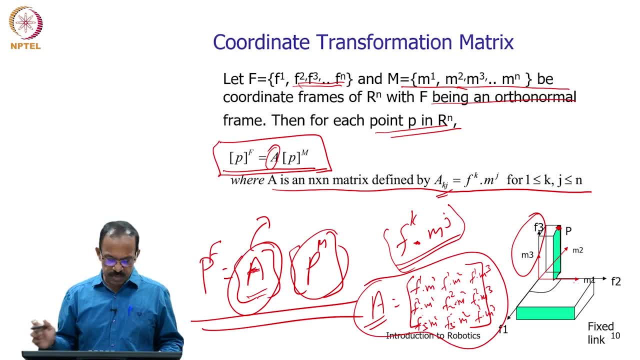 So the coordinate transformation between these two frames can always represented using a matrix A, and the elements of A can be obtained by taking the dot product of fk, dot, fk and mj. So you will be getting all the elements of the rotation matrix by taking the dot product. 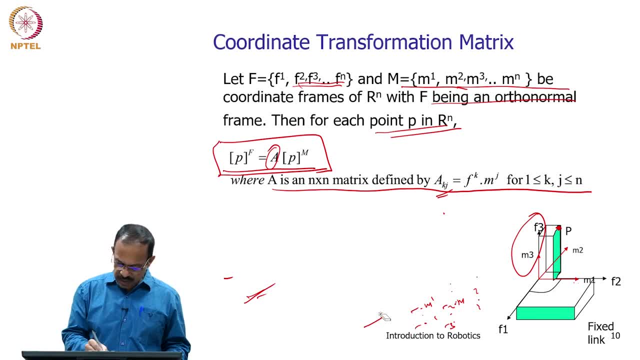 So that is basically the coordinate transformation matrix between two coordinate frames. So one is a fixed frame, another one is a mobile frame in this case. So the matrix A is known as the coordinate transformation matrix and A is given as f1. 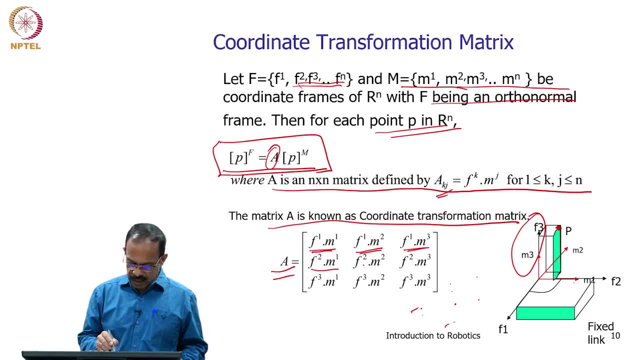 dot m1, f1 dot m2, f1 dot m3, similarly this one also. So this is known as the coordinate transformation matrix. So now, if you can, if you know the point P in mobile frame, Okay. 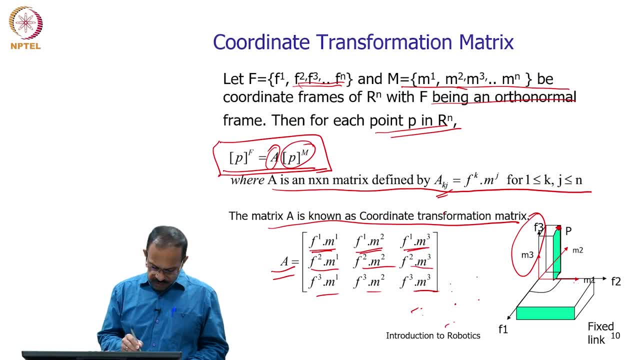 And you want to find out P, f. so what you need to know is what is A? and this A depends on how it is actually rotating with respect to the fixed frame, how the coordinate frames are aligned. The coordinate frames are aligned, both f1 and m1, f1- m1, f2 m2 and f3 m3, they are aligned. 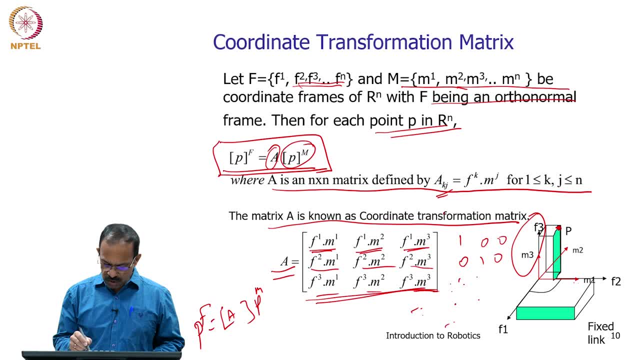 then this will be a 1 0 0, 0 0, 0 1 0, 0 0 1.. If f and m are aligned- For example, if this is f1, f2 and f3, and this is m1 and this is m2 and this is m3,, then 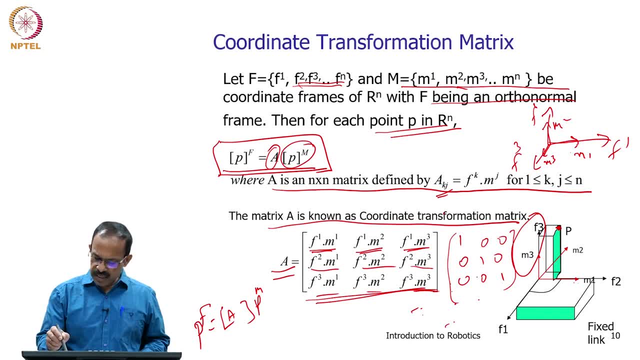 you will see that if f1 is aligned with m1, then f1 dot m1 will be 1, f1 dot m2 will be 0,. f1 dot m3 will be 0. Similarly, f2 dot m2 will be 1.. 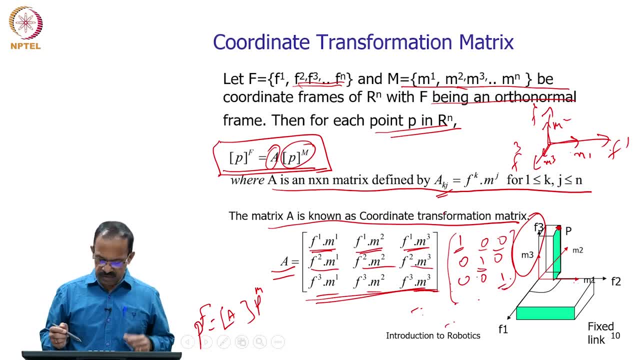 f3, dot m2 will be 1.. 0.. 0.. 1. dot M3 will be 1.. If they are aligned then the dot, the matrix will be 1 identity matrix and that it says that PF and PM are the same. So the point P in fixed frame and mobile. 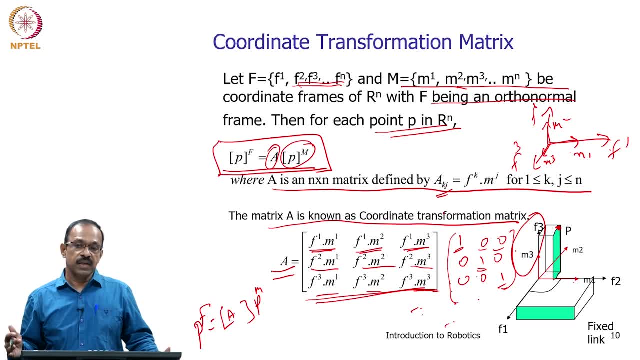 frame will be having the same coordinates. If they are not aligned, then there will be a different coordinates in the fixed frame and that is obtained by using this relationship. So that is what actually the coordinate transformation matrix. Hope you understood the coordinate transformation matrix. As I mentioned. some of you must be knowing all these things, But 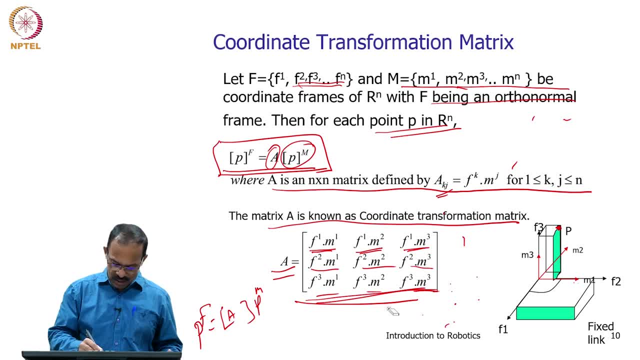 for those who are not familiar, I just wanted to ensure that you understand the basic principle of coordinate transformation matrix. Yeah, this transformation matrix is used in many other field also. Now, if you know this coordinate transformation matrix, then you will be able to understand. 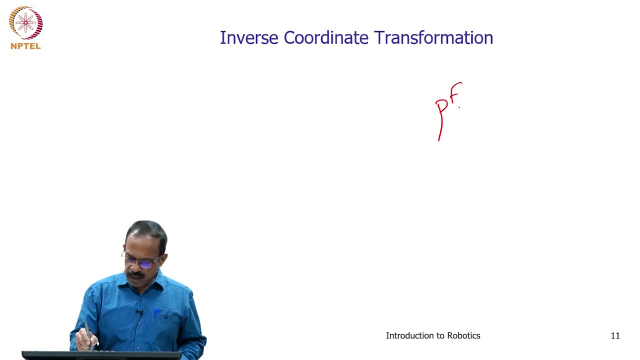 this coordinate transformation matrix. So that is basically we have PF is equal to APM, But we can do the inverse also. If we know PF, then we can actually find out PM from PF. So what we need to do is to use the A inverse So we can actually take the. 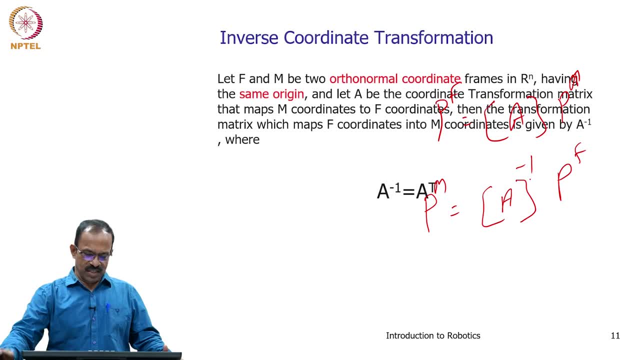 inverse of the coordinate transformation, provided the origin are the same. That is the only reason here. So we can actually get the inverse. I mean inverse can be obtained as a transpose in this case. So if F and MM, the orthogonal coordinates, are n having the 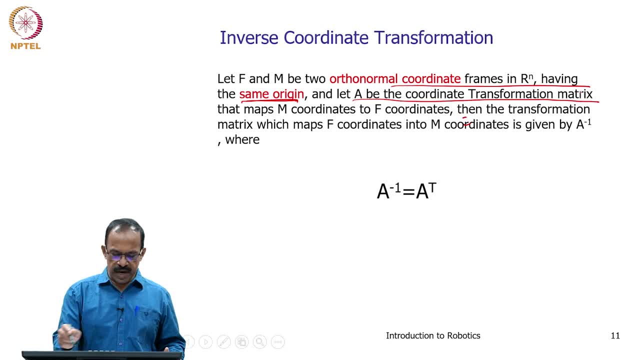 same origin and let A be the coordinate transformation matrix that maps M coordinates to F coordinates, then the transformation matrix which maps F coordinates to M coordinates is given by A inverse, where A inverse is equal to A transpose. So if you know A, you can use the A transpose to get the inverse coordinate transformation. 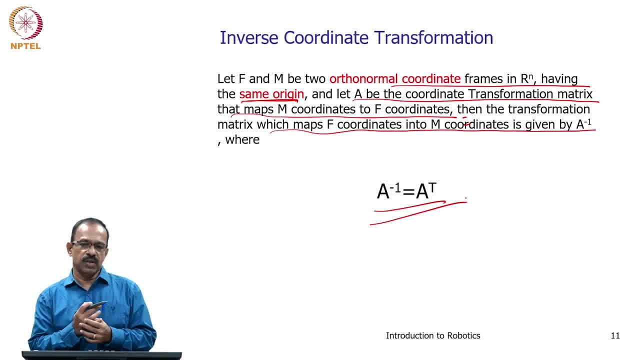 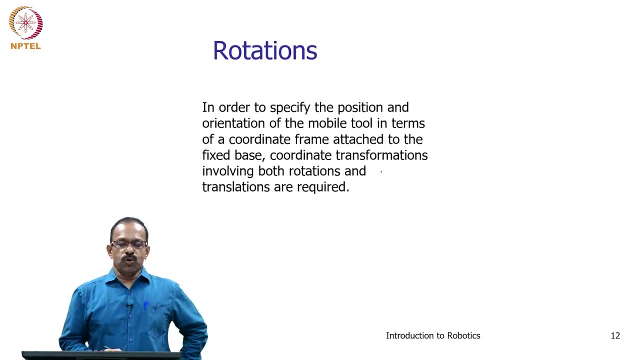 provided both the frames are at the same origin, So both having the same origin, then we will be able to use A inverse equal to A transpose. So that is the inverse coordinate transformation matrix. So that actually talks about the basic principle of coordinate transformation, That is you. 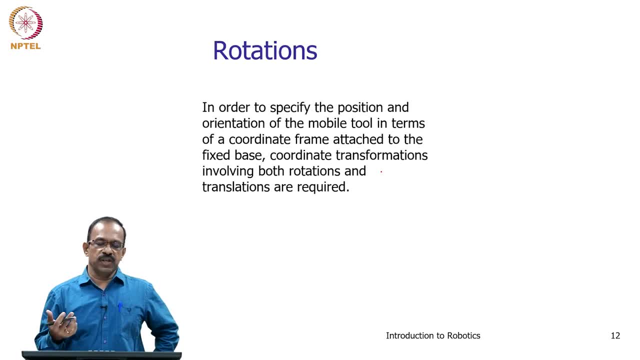 have two coordinate frames and you want to represent a point with respect to one coordinate frame from the other frame, Or you know one, the point with respect to one coordinate frame. the coordinates are known. you want to know the coordinates with respect to the other frame, So one we call. 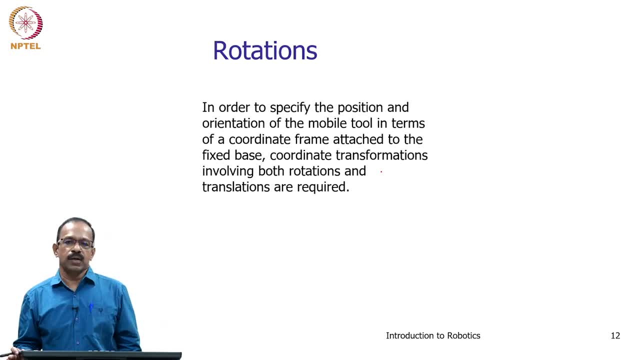 it as fixed and one we call it as mobile. If the frames are moving relative to each other, then we will be able to get the coordinates by using the coordinate transformation matrix, And what we need to do is to take the dot product of the axis and get the matrix. you 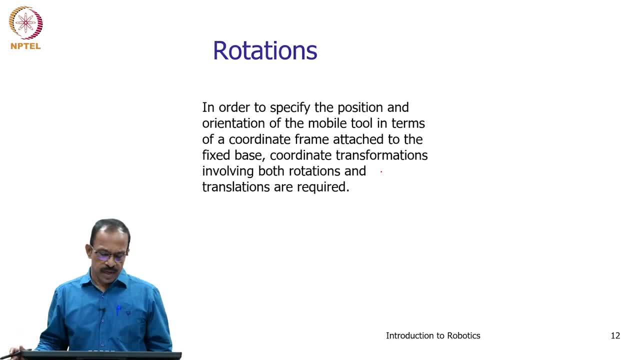 will get the coordinate points. Now let us consider some of the transformation, because we know there is a movement of the frame- mobile frame- So let us consider some of the movements. So, for example, if you have a frame like this, a fixed frame, F1, F2- 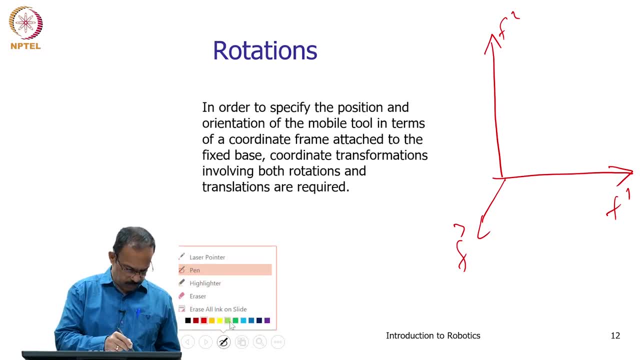 and F3.. Now I will define a M1, M1, M2 and M3.. So this, these two frames, initially they are aligned, they have the same origin. So there can be two ways. it can actually transform or it can move two ways. 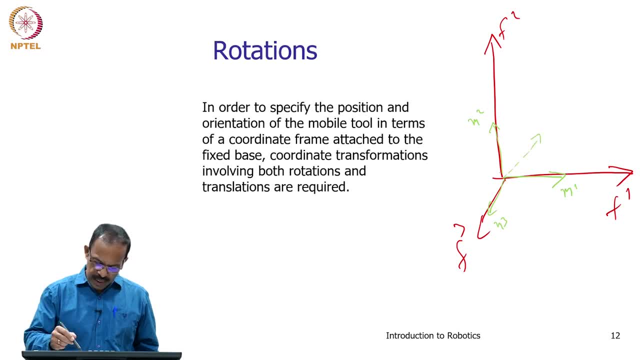 One is that it can actually rotate. the mobile frame can actually rotate. M1,, M2, it can actually rotate. assume that it is rotating with respect to M3.. So you will be getting this as M1, the new M1 will be this and this will be the M2.. So that is one. so, basically, we are saying: 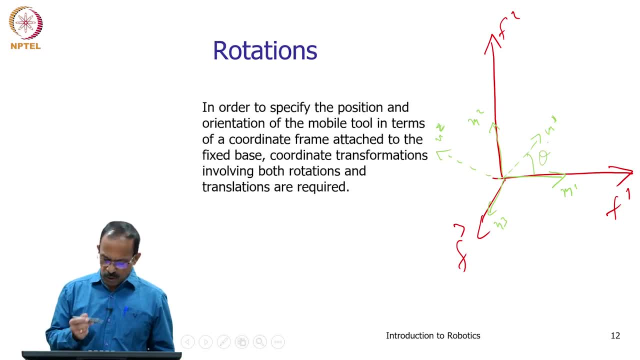 that the coordinate frame is rotated by an angle- theta- with respect to F3 or M3. So that is one way of rotation. one way of rotation. So this is the moving movement, And another one is that the transformed one. you can actually 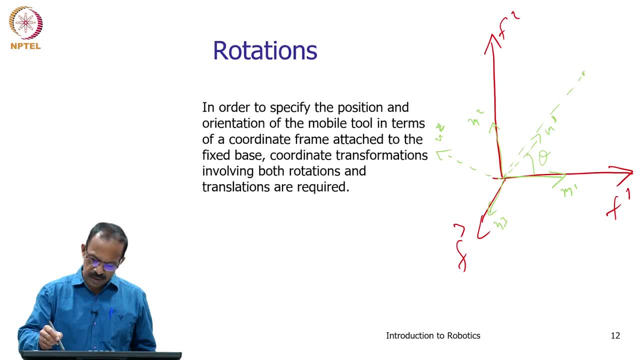 move somewhere here it can actually translate. it can translate and then assume that it is initially translated, like this M1, M2, and then it can actually rotate also. I mean, you can have a translation rotation or rotation translation, anything like that, is possible. 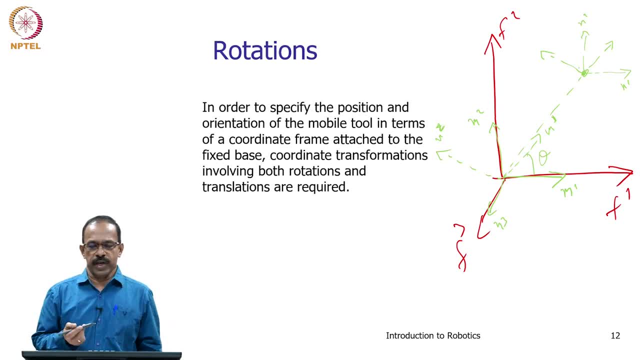 So there are multiple ways in which the coordinate frame can move, or an object can move or a moving object can move. So there are multiple ways in which the coordinate frame can move or it can move. So when you say coordinate frame is moving, you are saying an object. 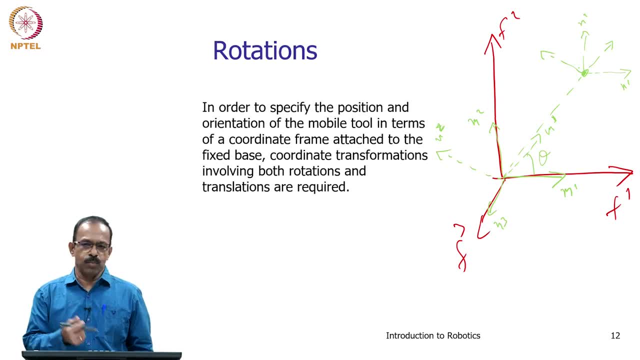 is moving and the coordinate frame attached to the object is basically the mobile frame. So the coordinate frame can actually have a rotation or it can have a translation of P. I can say this coordinate frame has moved from here to here and then rotated also. So 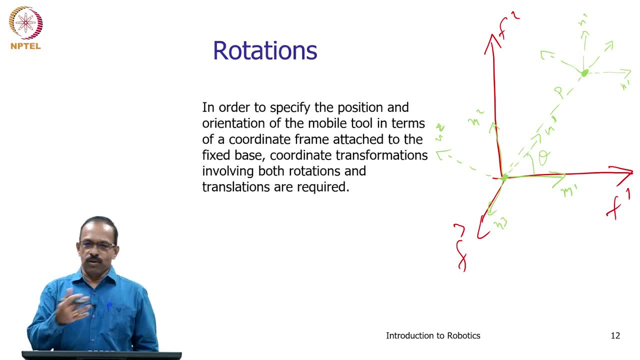 you can have a translation rotation or you can have a rotation and translation. So there are different ways of moving. So we first consider the rotation only. we consider that the coordinate frame is rotating. and when it is rotating we are interested to know: 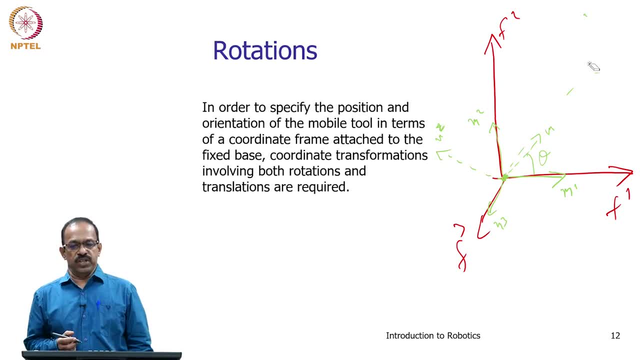 what is the transformation matrix when there is a rotation or there is a pure rotation? So we want to specify the position and orientation of mobile tune in terms of coordinate frame attached to this. So normally the transformations involve both rotation and translation. So 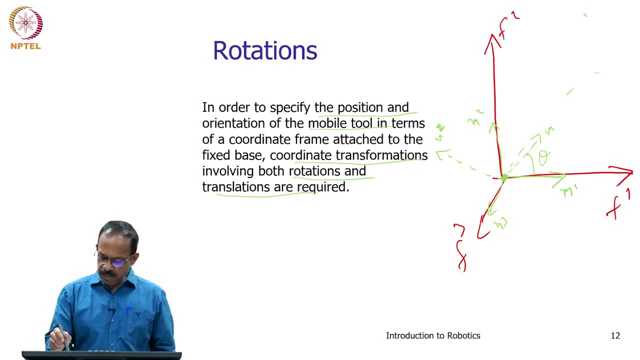 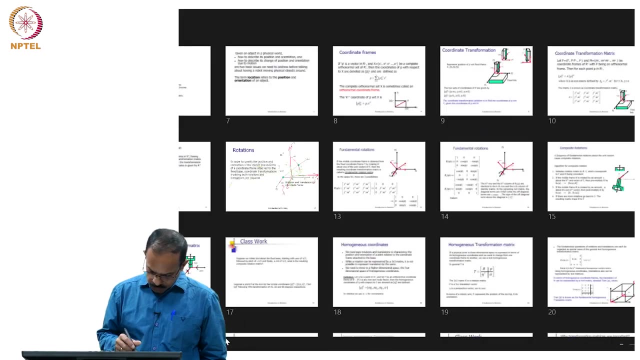 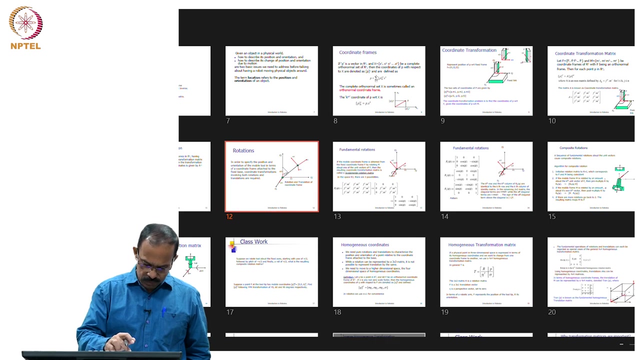 first we consider the rotation alone. that is, this mobile frame has rotated by an angle- theta- with respect to the fixed frame and we want to find out what is the transformation matrix. So we know that P f is. we know P f is a Pm, So we can see that a Pm is theVerb. Now 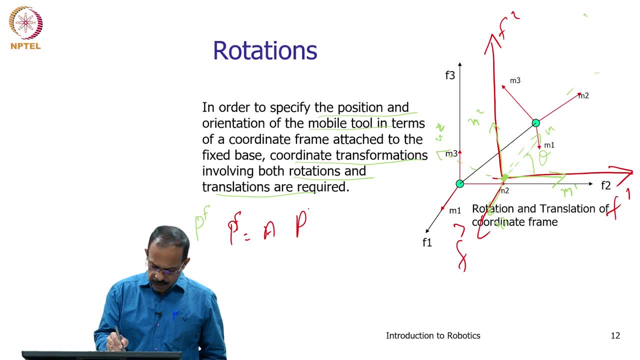 all the program can tried ovals, it is now P multiplies, it is now fatigue. So we are returned to the fixed frame and we want to know the transformation matrix. So we know that Pf is roommates. So now we know pf is a Pm. So it estamos debieled, we search. 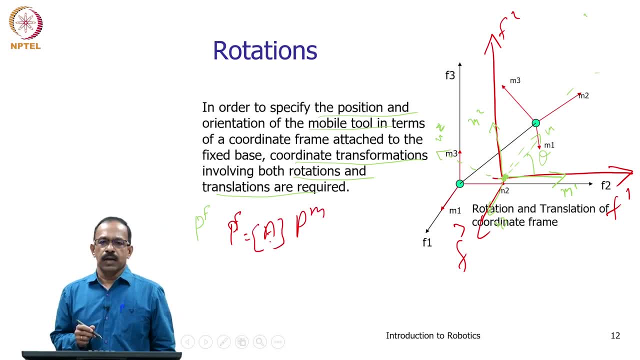 straight sub frank, Declaring separating out two of the platforms. there are states of And A is the transformation matrix. Now, we want to find out what is this transformation matrix when there is a rotation. That is, you want to find out what is this A when there is a rotation, and we know that. 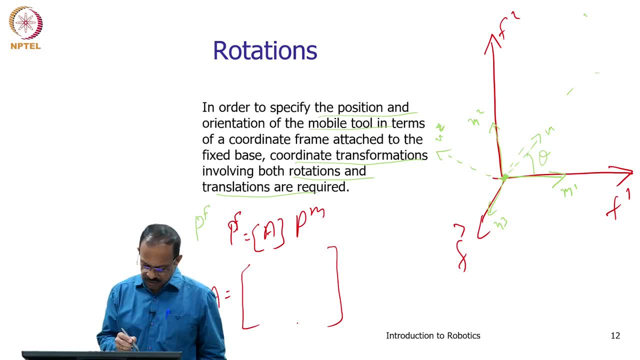 this rotation matrix. sorry, the transformation matrix is defined as F1 dot M1, F2 dot M2, sorry. F1 dot M2, F1 dot M3, similarly F2 dot M1, F2 dot M2, F2 dot M3,. similarly F3. 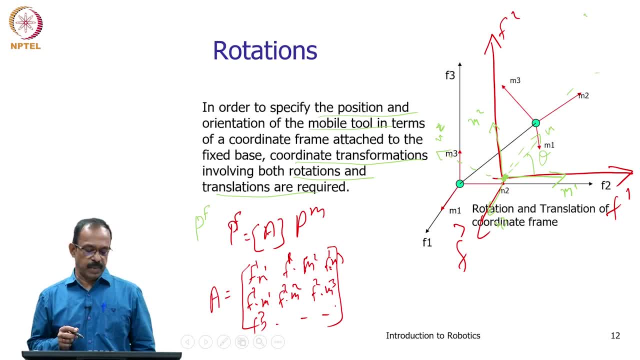 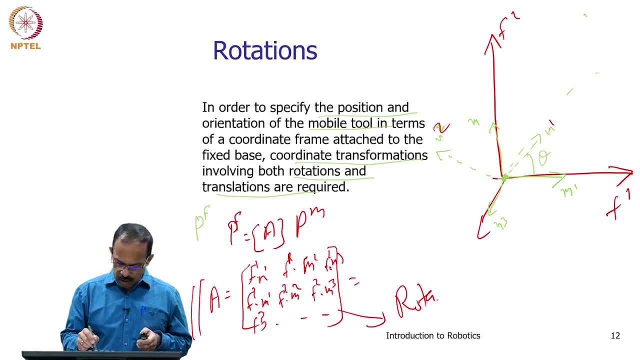 also. So this is the way how the rotation matrix is, this matrix is defined. So first, if it is only rotation, then we call this as a rotation matrix. so we call this as a rotation matrix. So we will look into this as a rotation function. 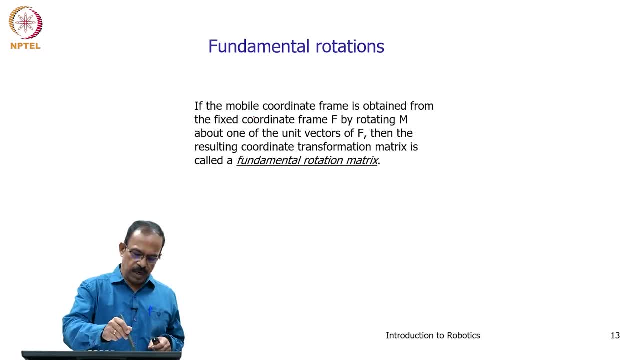 So fundamental rotation. so we will say that there is only one rotation. if the mobile coordinate frame is obtained from fixed coordinate frame by rotating M about one of the unit vectors of F, then the resulting coordinate transformation matrix is known as fundamental rotation matrix. 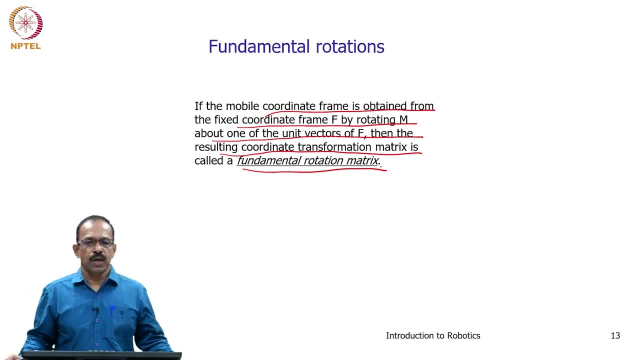 So if you have a rotation of the mobile frame with respect to one of the fixed frames, then we call this rotation as a, the transformation as a fundamental rotation, and the transformation matrix is known as fundamental rotation matrix. So, as I showed you, you can actually have a rotation like this. 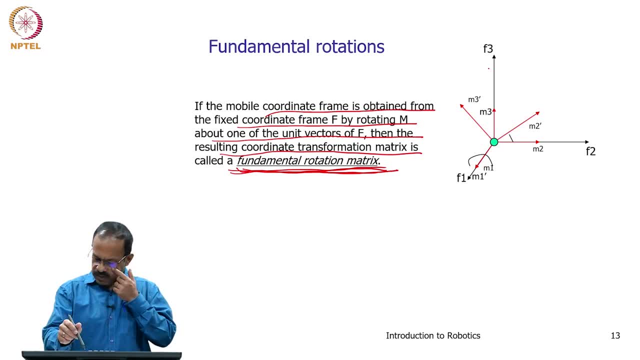 So you have F1, M1,, F2, M2,, F3, M3, that is, the coordinate frames can be F and M. So F1, F2, F3 represents the fixed frame and M1, M2, M3 represents the mobile frame. and then assume: 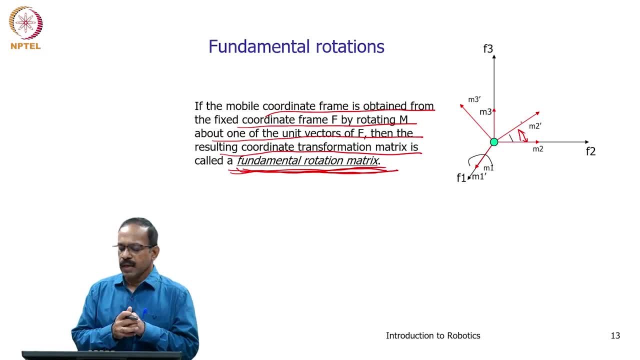 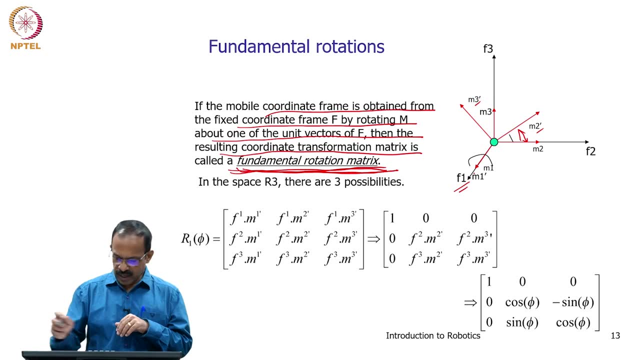 that the mobile frame has rotated by an angle, theta. now the new frame is M2 dash and M3 dash. So with respect to F1, it has rotated. we can get this as okay. so you can get this as R1 phi, as the rotation matrix, as F1 dot M1, F1 dot M2, F3 dot M3, like this F1 dot. 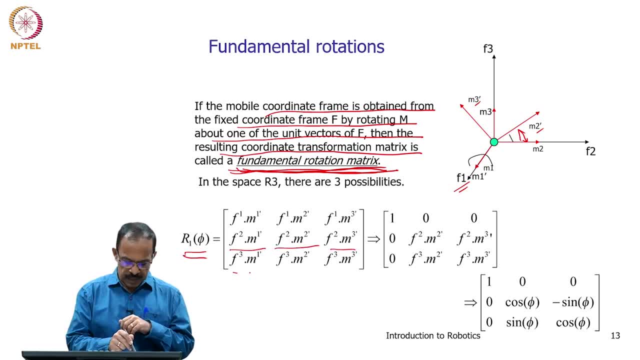 M3 and then F2 dot, M1 dash, M2 dot, F2 dash, like this. So we are actually taking the dot product of the rotated frame, rotated axis with respect to the fixed axis, and trying to find out what is the dot product. 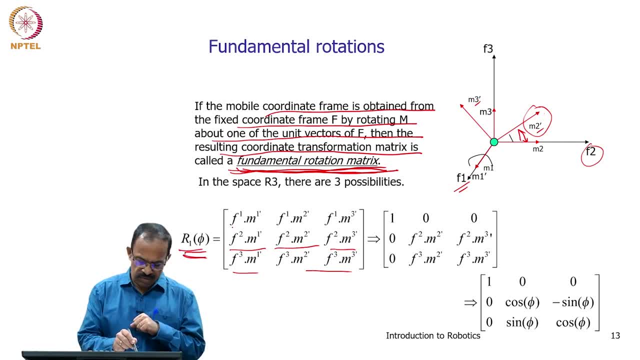 So this R1 phi or the fundamental rotation matrix, So we are actually taking the dot product of the rotated axis with respect to the fixed frame and then assume that the rotated axis is F1 dot M1 dash. Now we can see that F1 dot M1 dash. 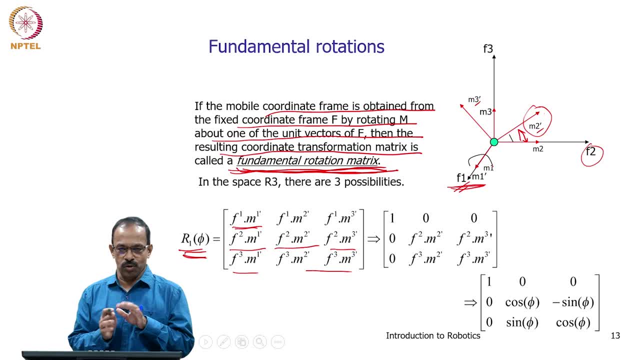 So this F1 and M1 dash are aligned. there is no rotation and there is actually. the rotation was with respect to this fixed frame. F1, and therefore M1 did not move and therefore you get this as 1.. So F1 dot M1 dash is 1, in this case, fundamental rotation, and this will be 0, 0, and this is. 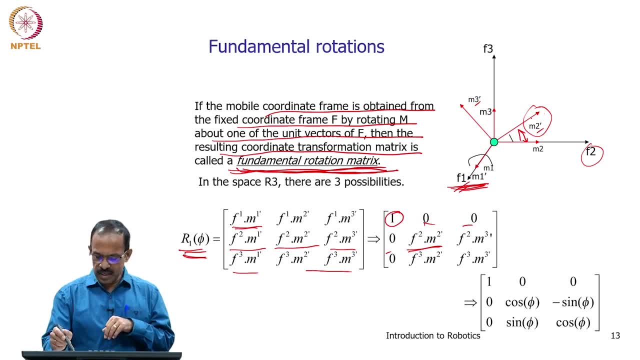 F2 dot M2 dash. So F2 and M2 dash, they are not aligned. they are not aligned, So there will be a dot product: F2 dot M2 dash, F2 dot M3 dash, F3 dot M2 dash and F3 dot M3 dash. And so this is 1 0, 0 cos phi minus sin phi this. 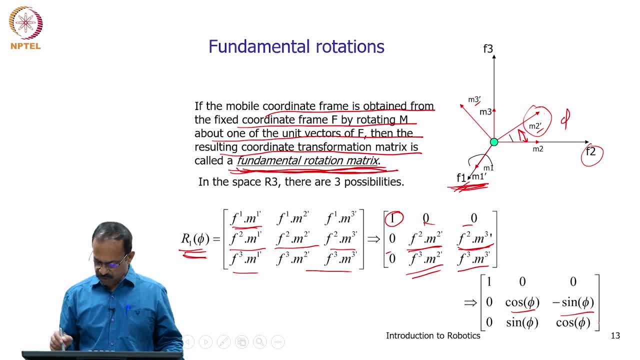 is by an angle phi. So you will get this cos phi minus sin phi, sin phi, cos phi. So this is the fundamental rotation matrix and the rotation is with respect to F1.. So when the rotation is with respect to the first axis, then the rotation matrix is 1, 0, 0, 1. 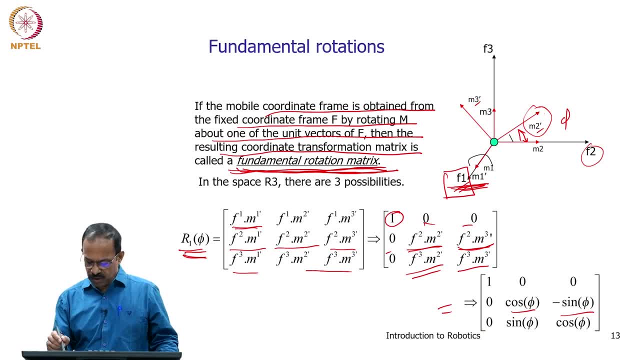 0, 0 cos phi minus sin phi, sin phi, cos phi. So this is how you get the fundamental rotation matrix. So whenever there is a rotation of the mobile frame with respect to the first axis of the fixed frame, your transformation matrix will be like this, and that is known. 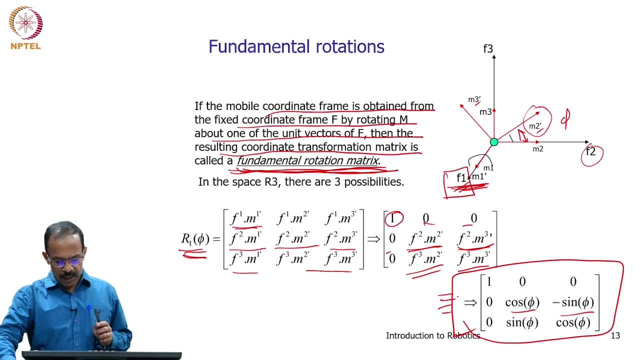 as the fundamental rotation matrix. So same way we can actually find out if the rotation with respect to F2 or the rotation with respect to F3, you will be able to get the rotation matrix. In the same way the difference will be: if it is rotation with respect to F2, then F2. 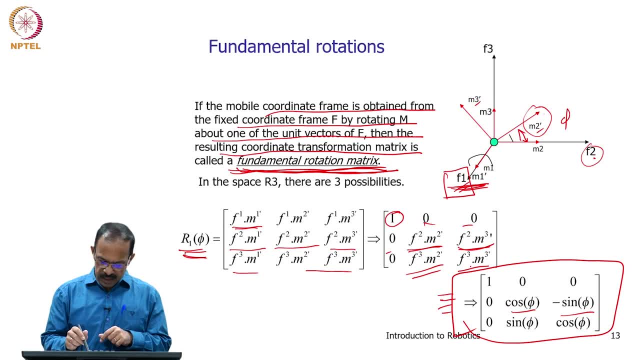 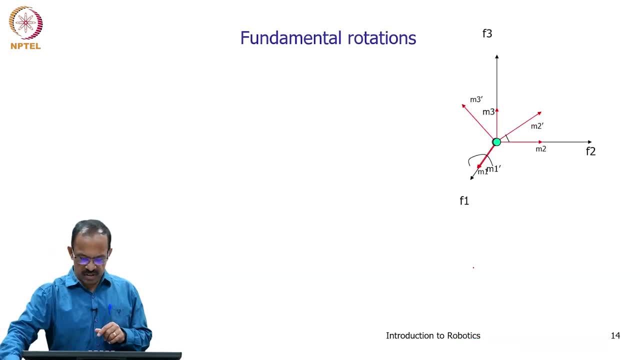 M2 dash will be 1.. If it is rotating with respect to F3, then this will be 1.. Otherwise the rotation, the matrix formulation will be the same. So you can get the fundamental rotations as like this: So R1, this rotation with respect to the first frame, first axis. 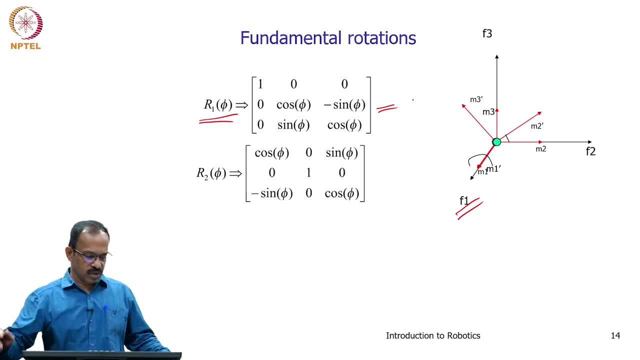 then this will be the rotation matrix. And if the rotation with respect to the second axis, F2, then this will be 1, 0, 0 cos phi minus sin phi, minus sin phi minus sin phi. So this will be the matrix. So you can see this will be 1, because F2 and M2 will be aligned. 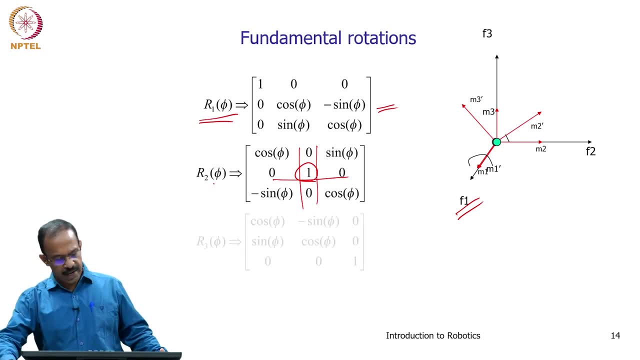 if the rotation with respect to F2 and the third one will be like this: R3 will be cos phi minus sin phi, sin phi, cos phi 0, 0, 1.. So the rotation with respect to the third axis. So this is the fundamental rotation matrix that you can identify whenever there. 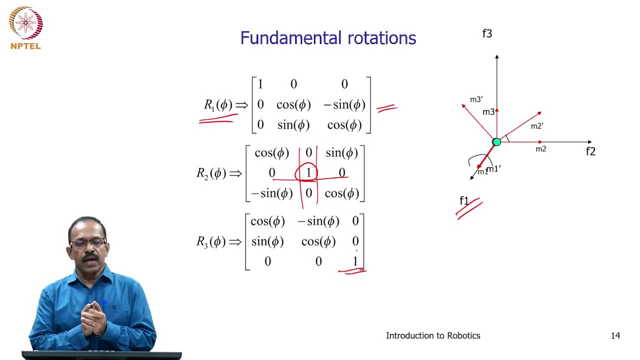 is a rotation of the mobile frame with respect to the fixed frame and the rotation is with respect to a particular axis, then you will be able to easily get that rotation matrix by using this rule. So first axis means the first row and first column will be able to. 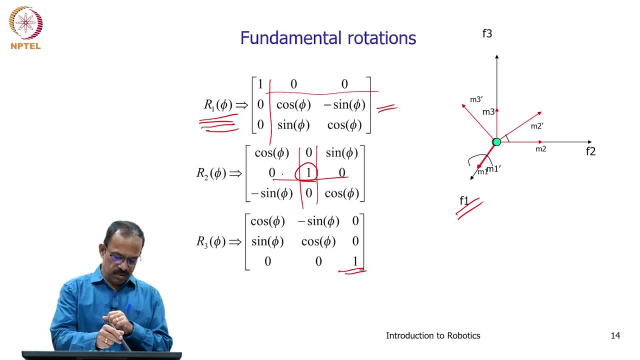 see like this: 1 0 0, 1 0 0.. Then this will be the second axis with respect to second axis, this one third axis, this one. So these are known as the fundamental rotation matrices or the transformation matrix, which represents only rotation. then we call it as fundamental. 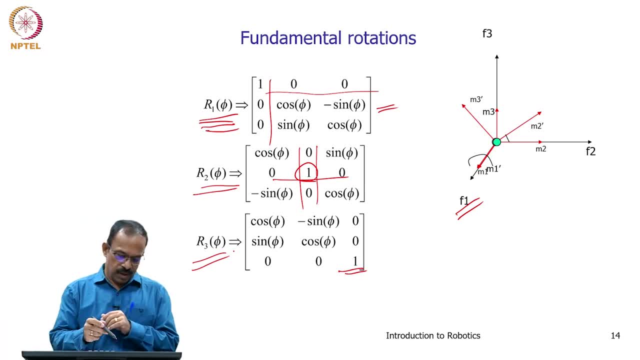 rotation matrix. Now, you do not need to really mean this will be. we will be using this many times in the kinematic analysis, but you do not need to remember it by heart. So there is a simple way to remember it. So there is a pattern in this one. So, if the rotation 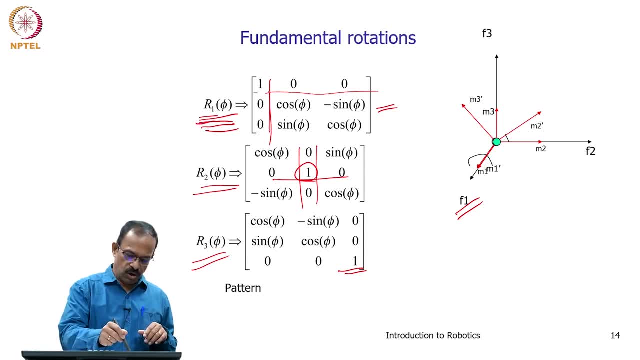 is with respect to first axis, you can see the first row and first column. first row and first column will be part of identity matrix: 1 0 0. 1 0 0.. If the rotation is with respect to second, then the second row and the second column will be integral. So this: 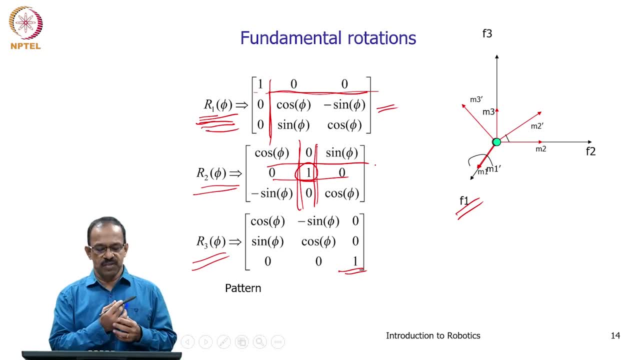 row and the second column will be part of identity matrix: 0 1 0, 0, 1 0.. Similarly, if the rotation with respect to third, third row and third column will be 0, 0, 1, 0, 0, 1,. 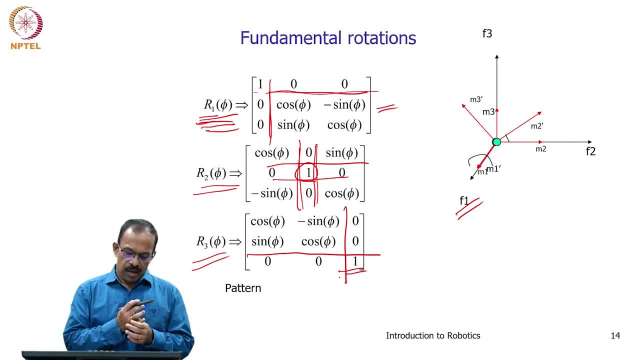 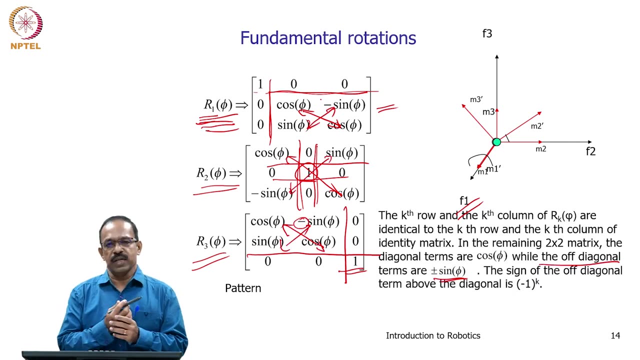 so that is the pattern in this, And then the diagonal will be always cos phi. see, this diagonal element will be always cos phi. So you can see, always it will be cos of diagonal elements, always will be plus or minus sin phi And the sin of the off diagonal above. 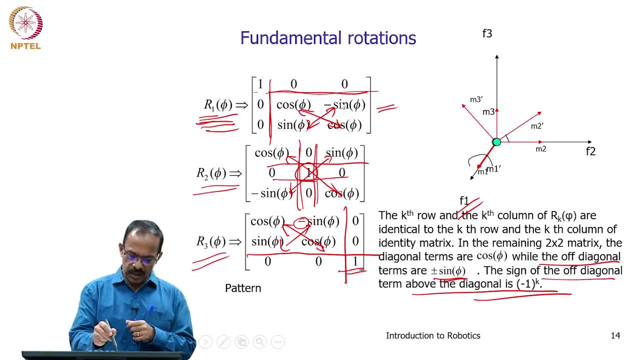 the diagonal is minus 1 to the power of k. So if you have a sin phi here and the sin of the off diagonal term above the diagonal is minus 1 to the power of k, So minus 1 to the power of k. so this is the above the diagonal is minus this one, so it is minus. 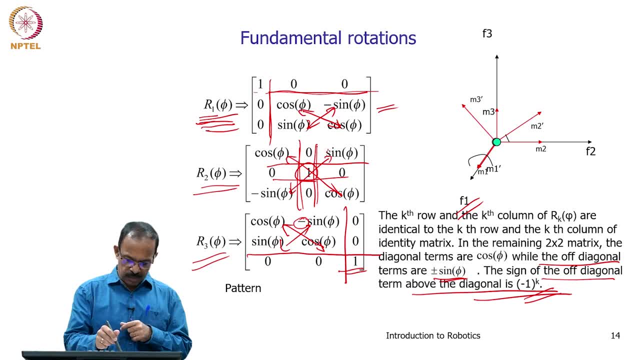 1 to the power of 1, this is minus 1 to the power of 2, this is minus 1 to the power of 3.. So you will get it as minus sin, minus, plus, minus. So you will always see that the k 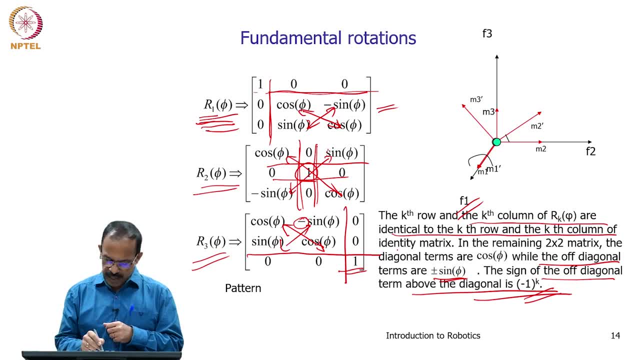 th row and k th column of R k phi are identical to the k th row and k? th column of identity matrix and the remaining 2 by 2 matrix. the diagonal terms are cos phi and the off diagonal always plus or minus sin phi. So it will be either plus or minus sin phi And the sin. 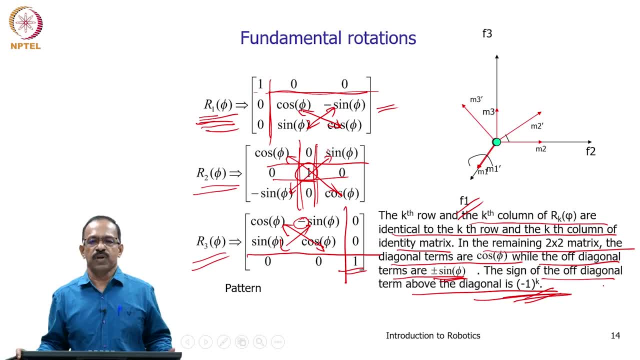 of the off diagonal term above the diagonal is always minus 1 to the power of k. So if you can remember this, you will be always able to get this So fundamental rotation matrix without any difficulty. So that is the fundamental rotation. 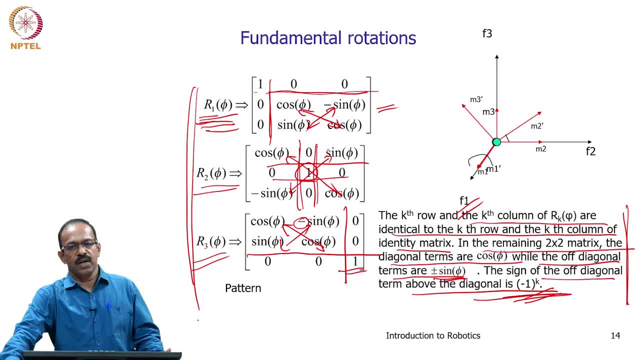 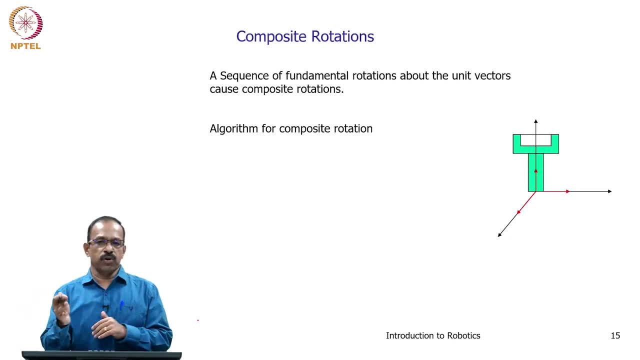 matrices when the mobile frame is rotating with respect to the fixed frame. Now suppose you want to get the composite rotations. Suppose you have multiple rotations taking place, because first this, suppose this is an object, and you have point P here, Now this red one. 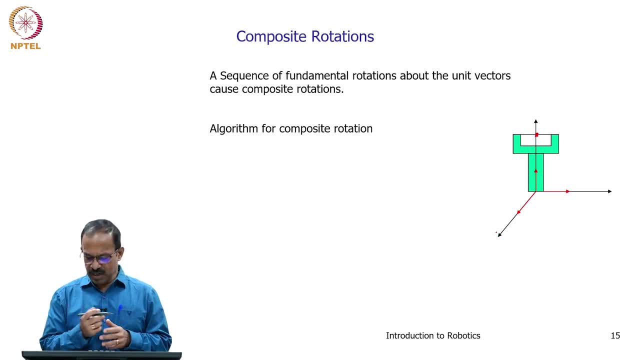 is the…. So this is the…. black one is the fixed frame and the red one is the mobile frame. assume that- and if you rotate it, you can actually see that this will be- you can be rotated in with respect to this axis, can be rotated with respect to this axis, then this will be moving to this side. 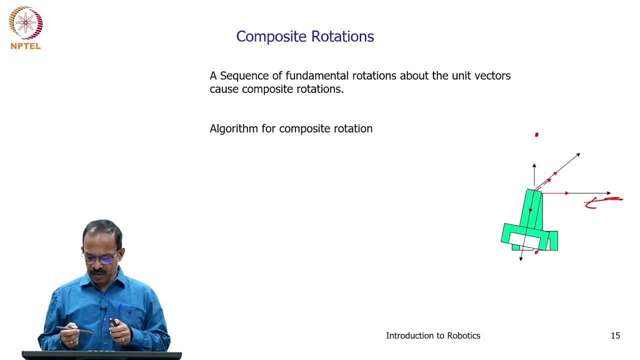 So you can actually get the P somewhere here and you can actually rotate again with respect to this. you can actually rotate with respect to the vertical axis. you will be getting this position as P. So, like this, suppose you have multiple rotations taking place. you want to? 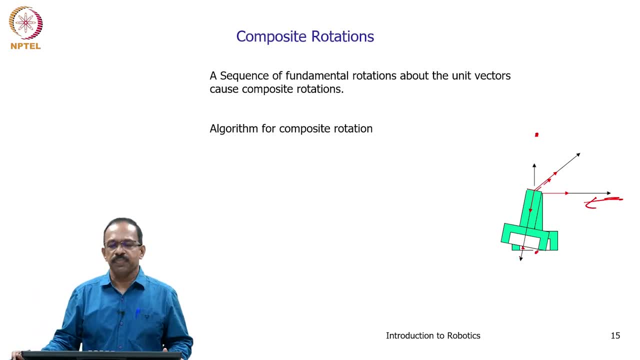 know what is the point of P, what is the point P with respect to the fixed frame? and this can be done by using a simple algorithm. So we need just need to follow a simple algorithm to get the composite rotation matrix, that is, initialize the rotation matrix R to I an. 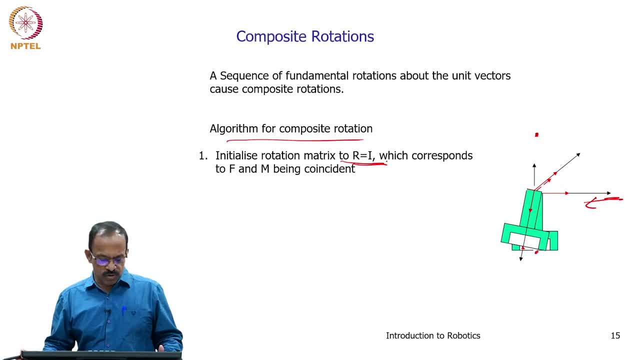 identity matrix which corresponds to F and M being coincident. So assume that F and M are coincident initially, and assume that your rotation matrix R is identity matrix And then look at the rotation if the mobile frame M is rotated by an amount phi about. 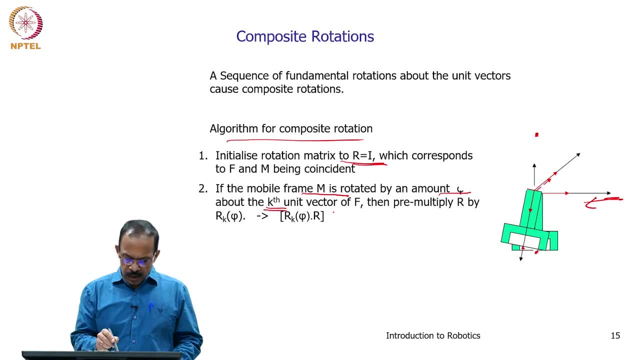 the kth unit vector of F, then pre-multiply R by R k, phi. So initially R is I. now you look at what is the rotation happening. if the mobile frame is rotated with respect to the kth frame of fixed frame, then do a pre-multiplication. then R is equal to I, R, k, R k, k is equal to. 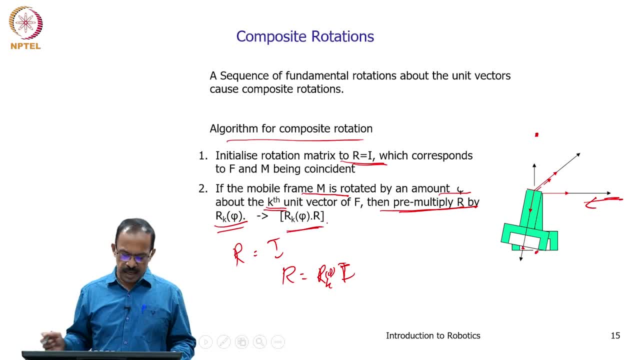 1, 2 or 3, so you can get this as a pre-multiplication: R k multiplied by R. that is R, so R is phi now. so it is R k multiplied by R, so new one. But if the rotation is with respect to mobile, 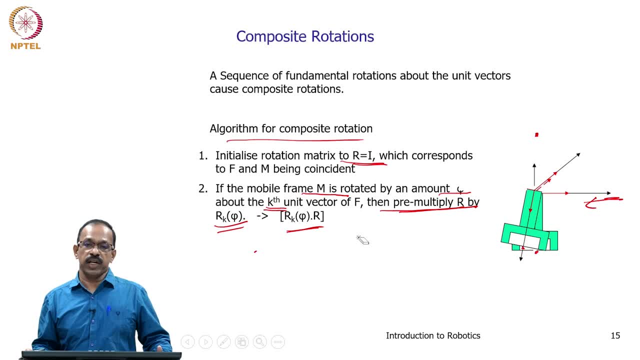 frame or its own frame, because the object can actually rotate with respect to its own frame also, not necessarily that it should always rotate with respect to fixed frame. it can rotate with respect to its own frame also, and that is. that is the case, then what you need to do is to a post multiplication. So here, if the rotation is with respect to 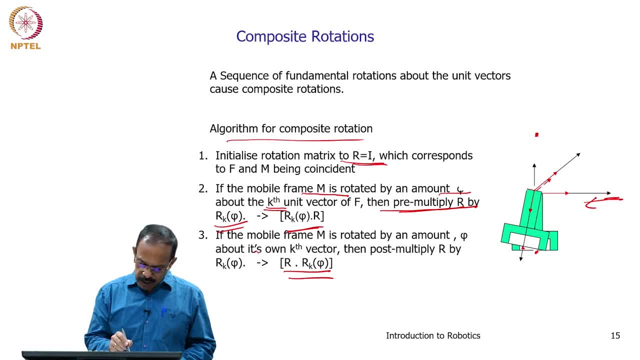 the kth vector of its own frame, its own kth vector. then you do a post multiplication, so then R is multiplied with R k. So the post multiplication and pre-multiplication makes difference and therefore the rotation can actually be represented using either a post. 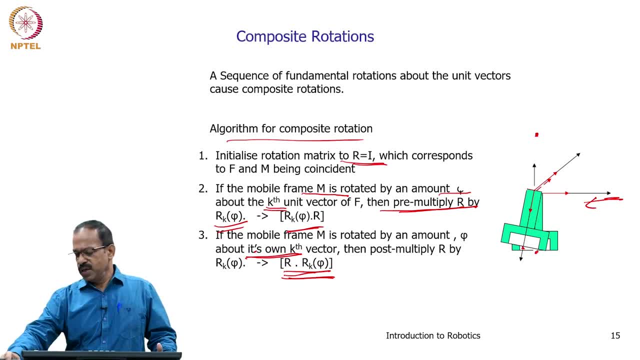 or pre-multiplication. So this is the algorithm that we need to use, and if you have more multiplication, more rotations, keep on doing this. keep on doing this till you complete all the rotations. So that is how you get the composite rotation matrix: by looking at whether it is rotating with. 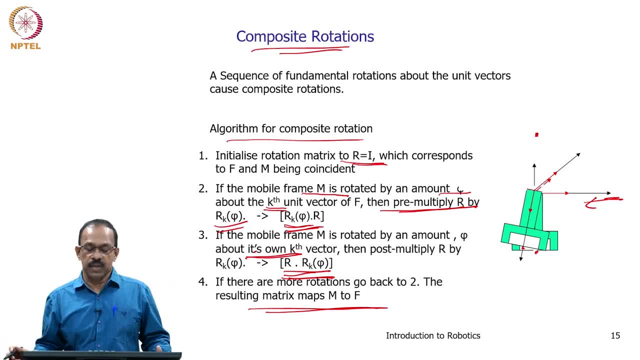 respect to its own frame, or with respect to the mobile, the fixed frame. You continue this till all the rotations are completed and the resulting matrix maps M to F. So you can get the M to F mapping by the resulting composite rotation matrix. So that is the way how you get the composite rotation matrix. So I will stop here. so we 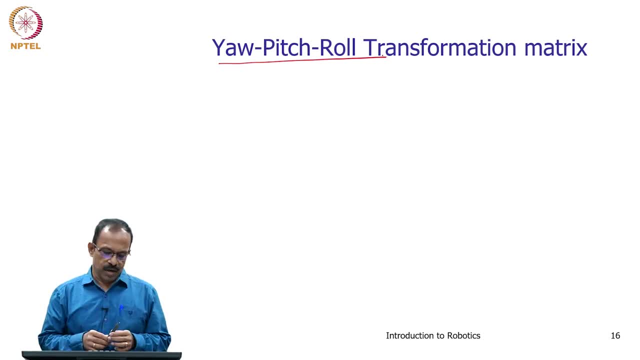 will talk about this Yaw pitch roll transformation matrix as a composite rotation and then we will see how to get the transformation matrix using the algorithm that we discussed. So we will discuss this in the next class, Thank you.